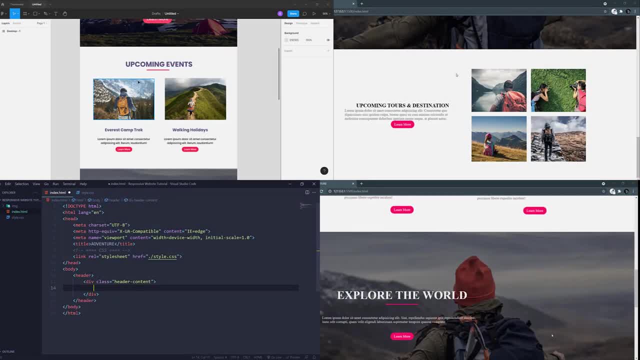 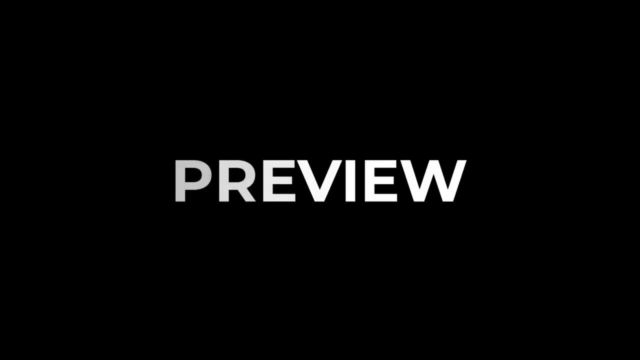 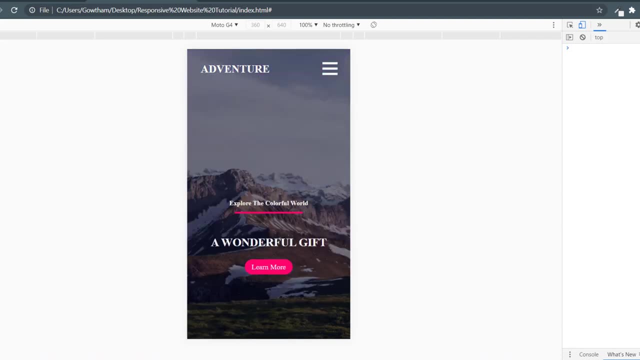 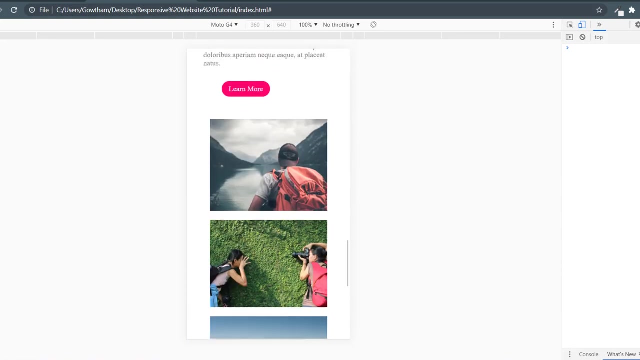 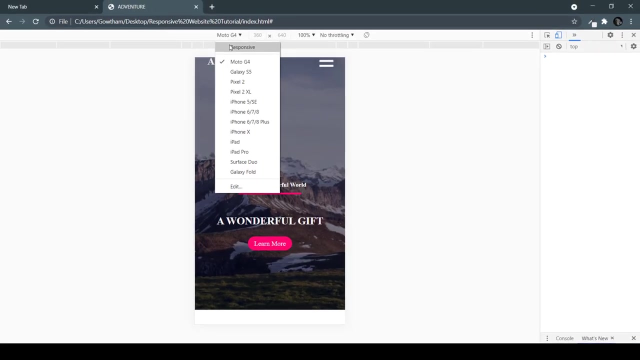 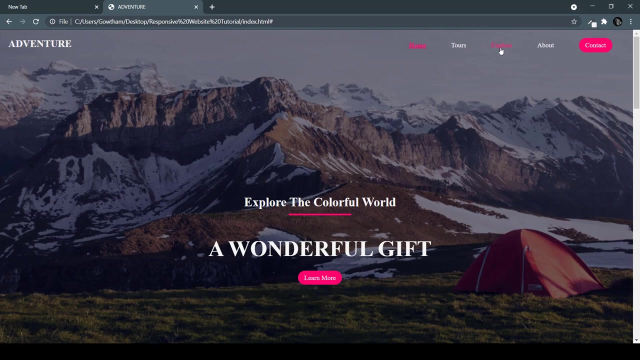 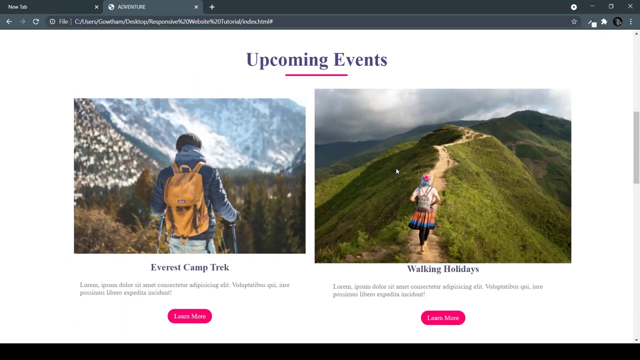 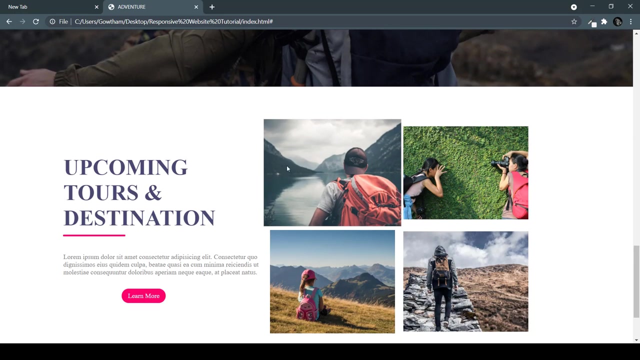 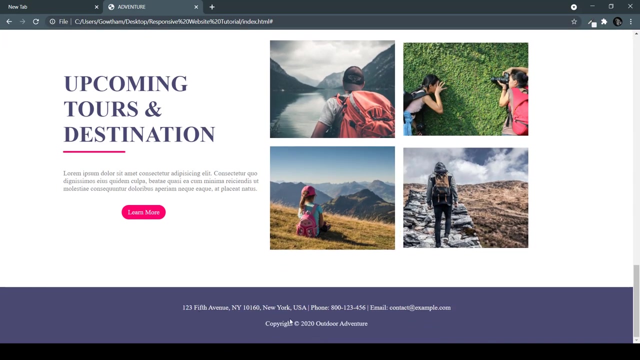 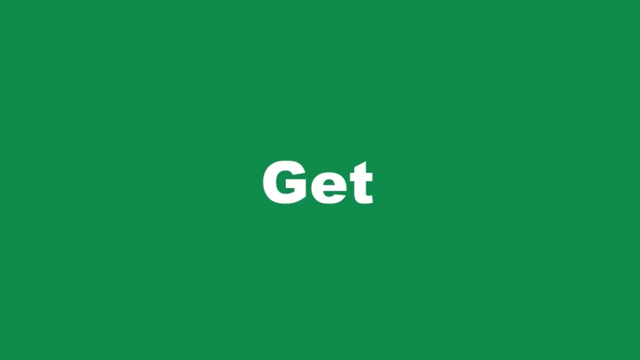 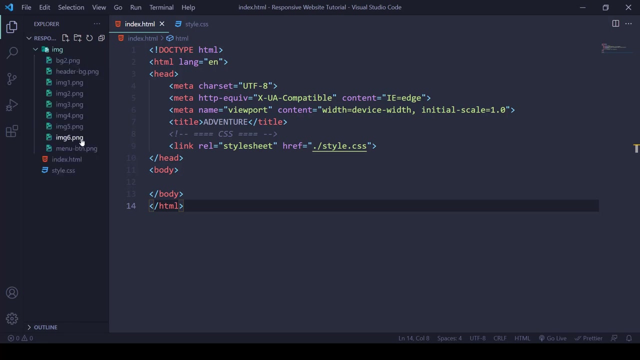 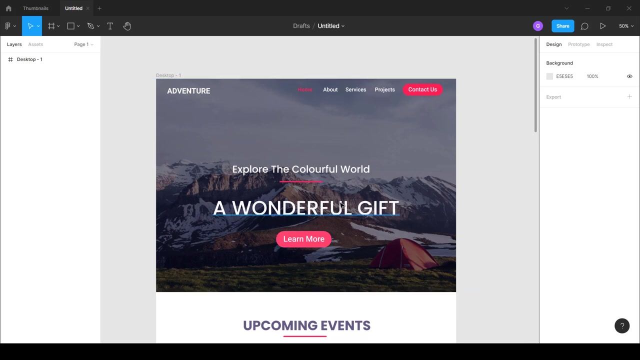 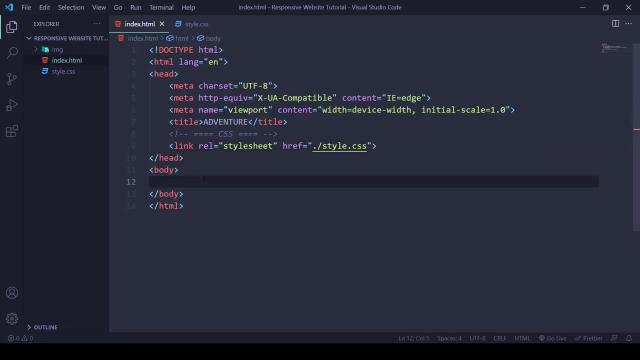 Hey guys, in this episode we are going to build this complete responsive website with HTML and CSS. Let's get started. Hey guys, in this episode we are going to build this complete responsive website with HTML and CSS. Let's get started. We have a header content and inside our header content we have a h2 with a text called explore the colorful world. 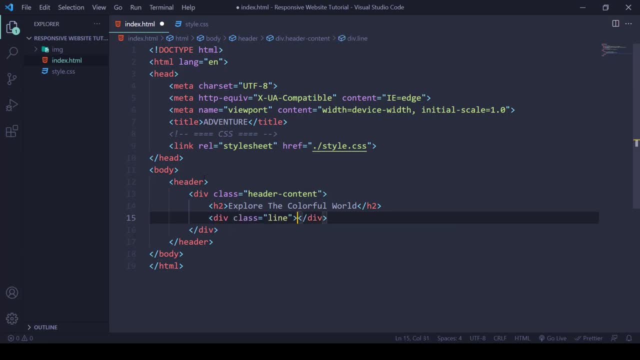 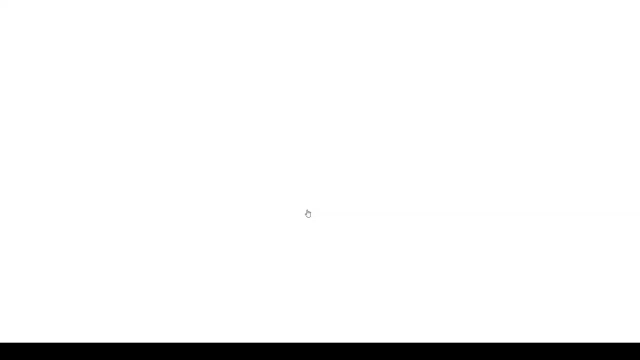 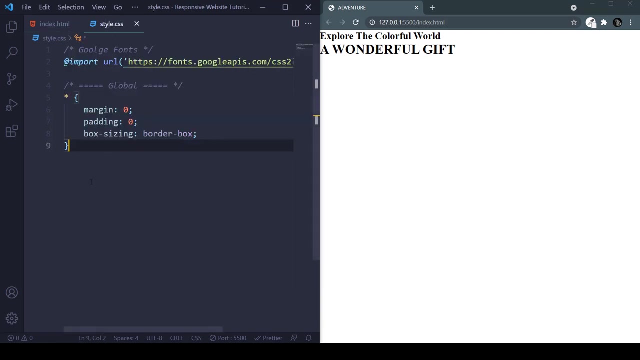 And after this we have a div called line and after that we have a h1 with a text called a wonderful gift. So now let's open this with live server. Now let's style this. So let's open our CSS file and inside this target our header and make width 100vw and height 100vh. 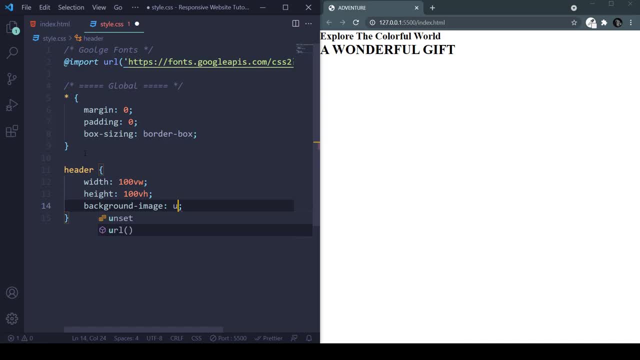 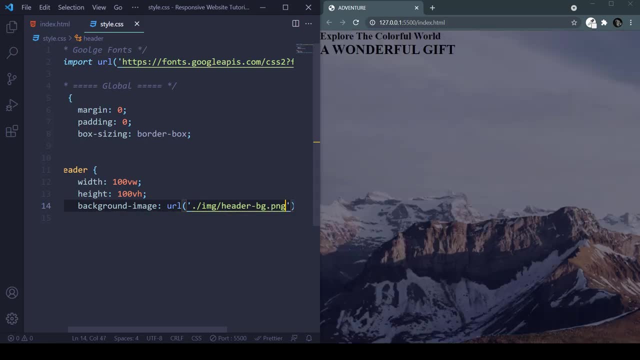 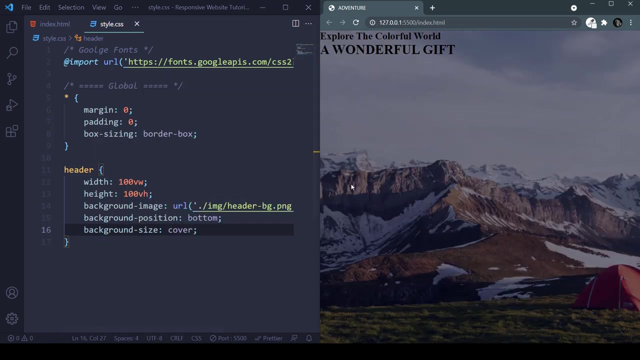 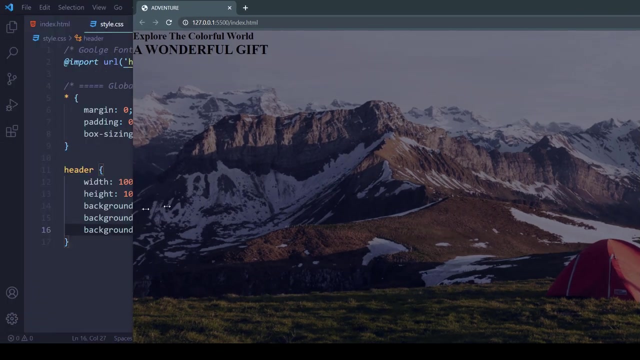 And add background Background image url inside our images header vg And make background position bottom and background size cover, You can see our beautiful full screen background image. You can see this is completely responsive. This image grows up when we are in desktop mode. 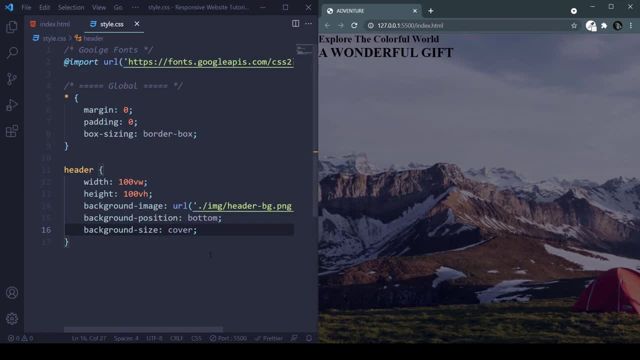 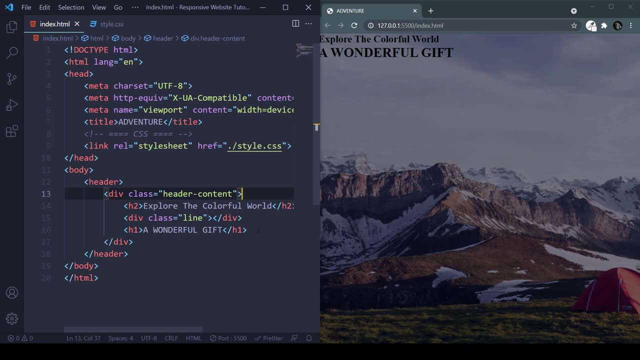 And it shrinks down to mobile devices as well. Now let's make this text into center, And before that let's add a button here, And after our h1 let's create an anchor tag with a class name of ctn. So we will learn more. 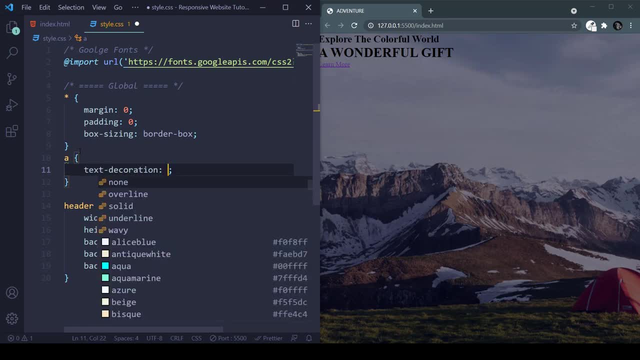 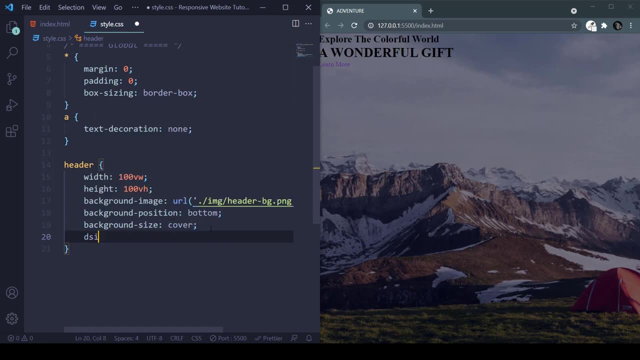 For all our anchor tags. remove text digression to none For our header. add display flex And align items. center and justify content center. Now we can see our text is in center right here, And if we make align items to end flexend. 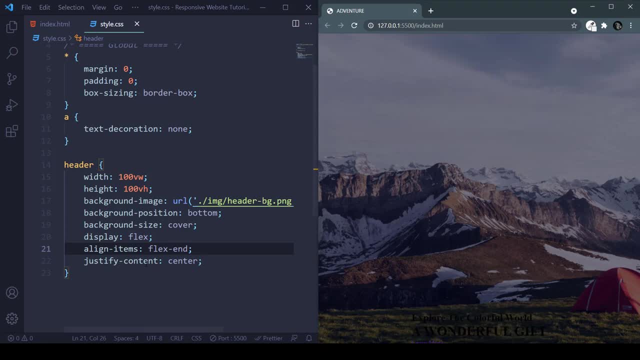 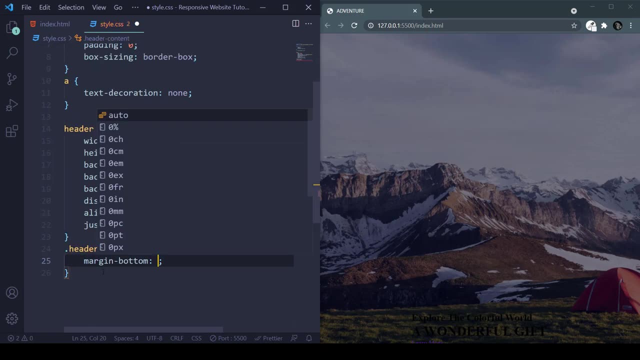 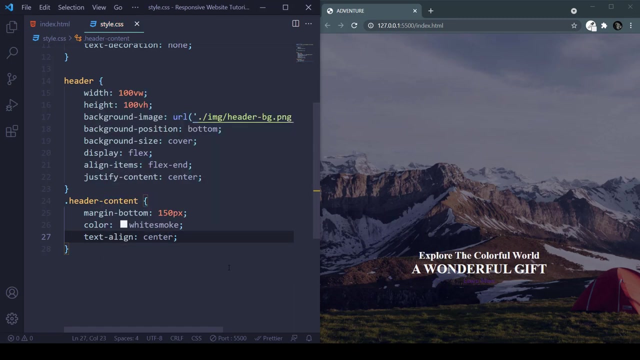 Our text will be right here. You can see our text to be here Now. let's target our header content And add in. We can see our text is here. margin bottom of 150 pixel and color: white smoke and text align center now. 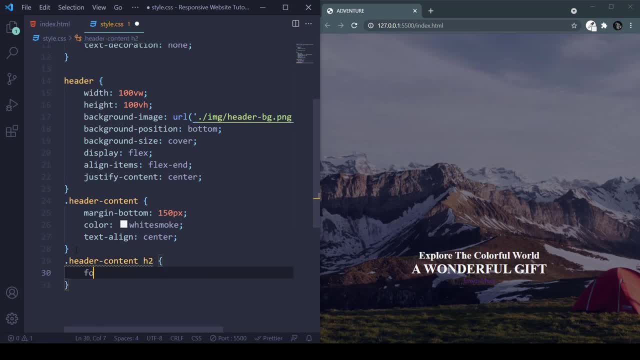 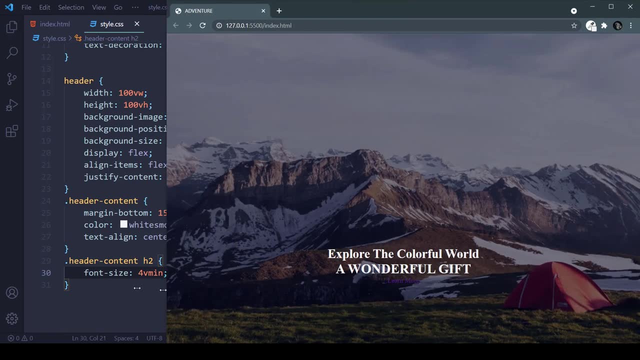 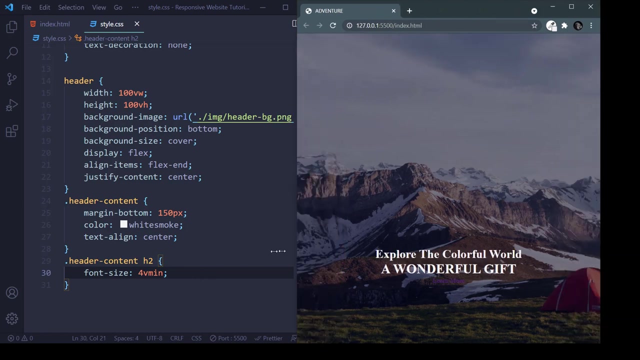 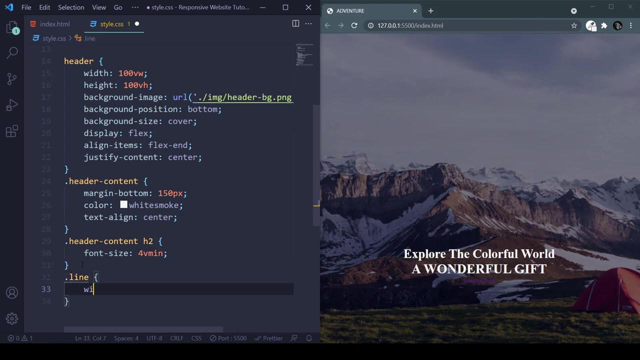 inside our header content. let's target our h2 and add a font size of 4 vmin. by adding vmin, our text will get responsive. if you see, if I increase the width, our text size increases, and if I decrease the screen width, our text size also decreases. and now let's target our line on this: add a width of 150 pixel. 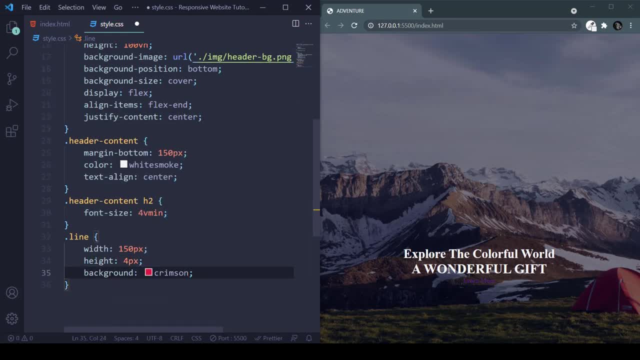 and a height of 4 pixel and add background of this color. and now you can see our line is at starting of the text. to make it into Center, add margin and top and bottom 10 pixel left and right auto. you can see our line is in Center. 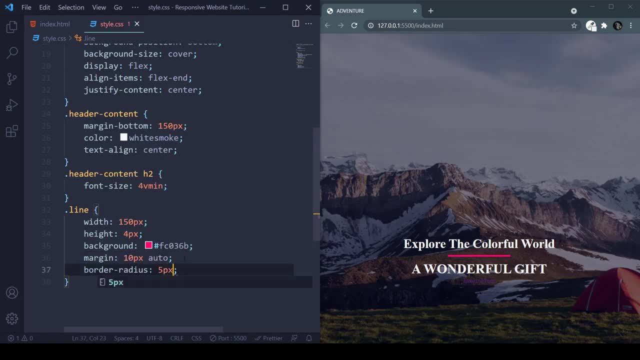 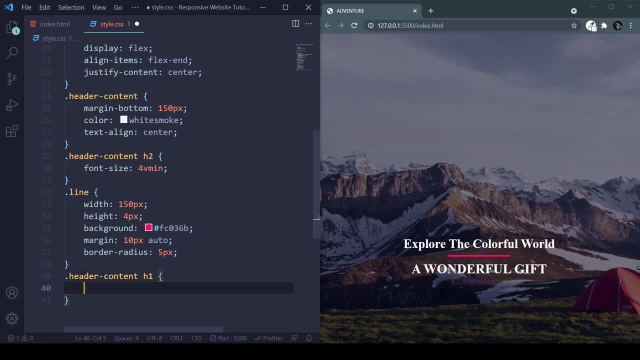 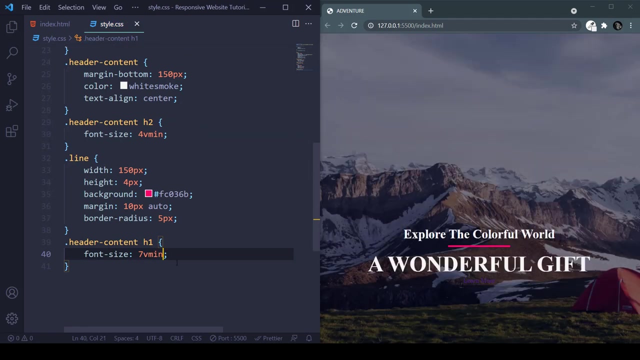 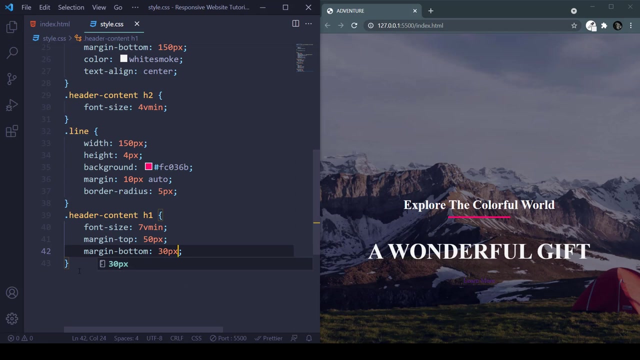 for this I had a border radius of 5 pixel. and now inside our header content, let's target our h1 for this, add a font size of 7 vmin and add margin top and bottom: 50 pixel margin bottom at the pixel. now let's target our CTN, which is: 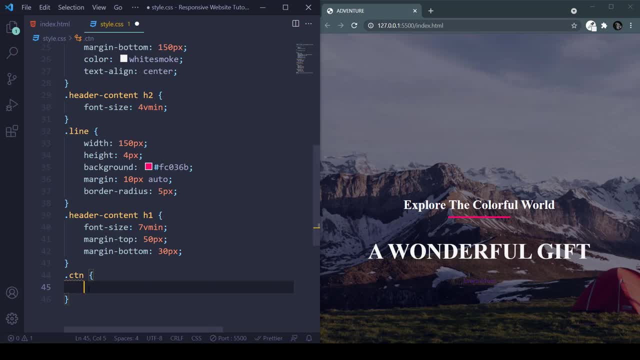 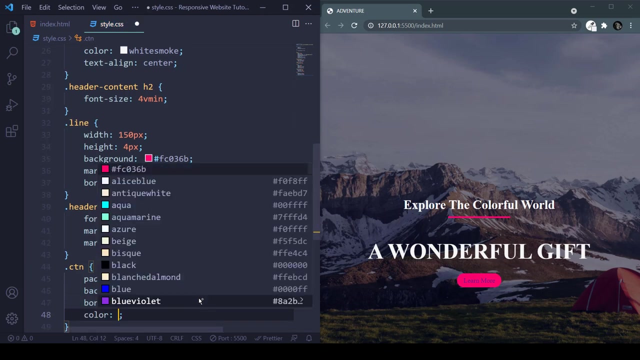 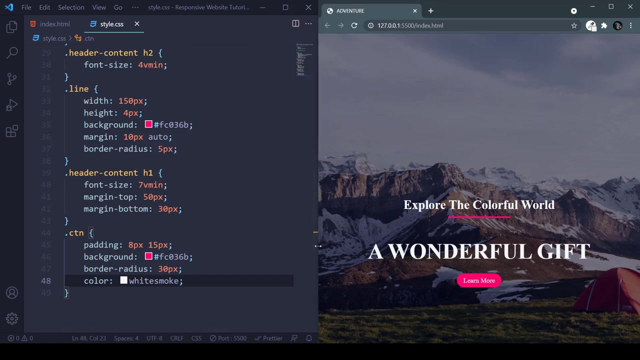 this lap more button for this. add a padding of 8 pixel top and bottom and 15 pixel left and right and add a background of this line color. make border radius 30 pixel and color white smoke. now I can see our beautiful full-screen background image is completed. I can see this is. 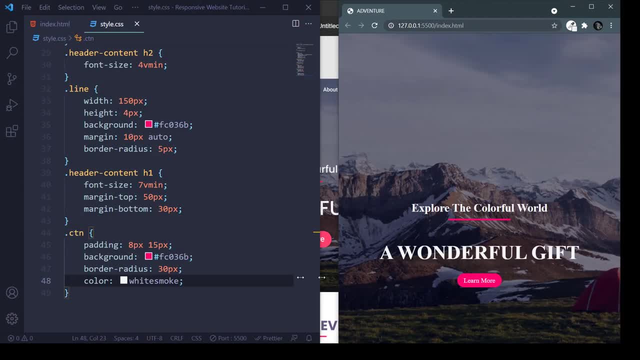 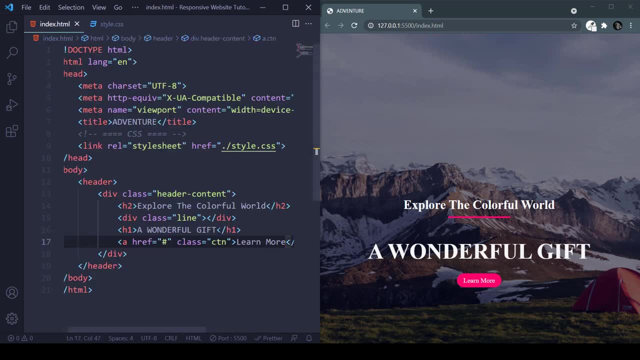 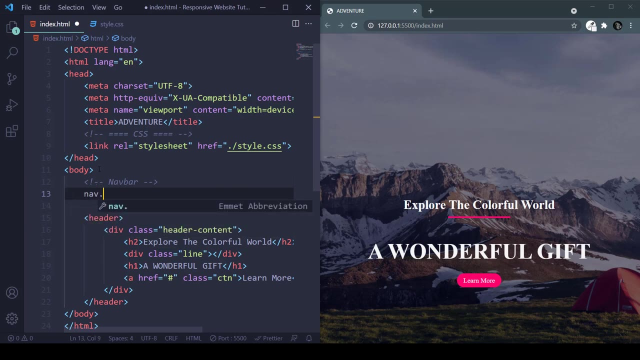 completely responsive. now let's move on to our network. so now let's open our HTML file and before this header, let's create our now. but I will create a now with a class name of now, back and then say that we have our logo, or logo will be: 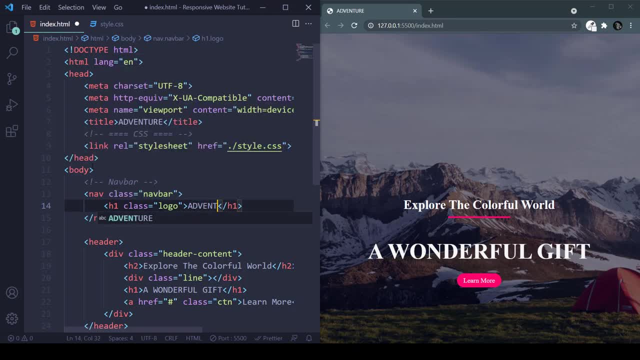 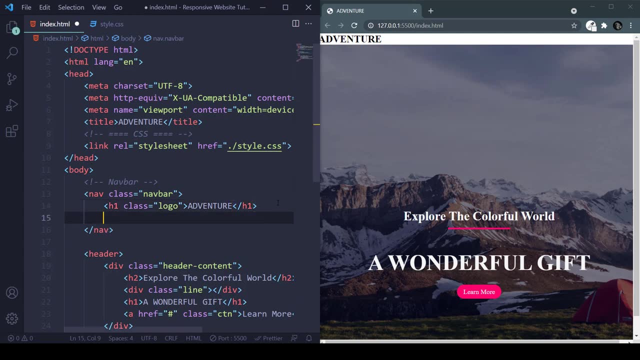 adventure you logo. we have a ul with a class name of now links inside that we have some allies. this is for home and if you hold alt, shift and down arrow, this will copy that line and i will copy this two more, three more times. this is for tours, this is for explore and this is for about. 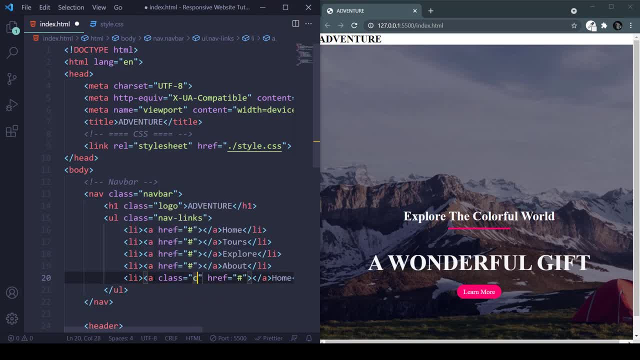 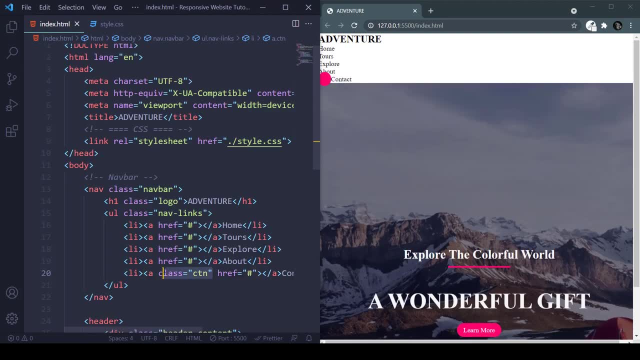 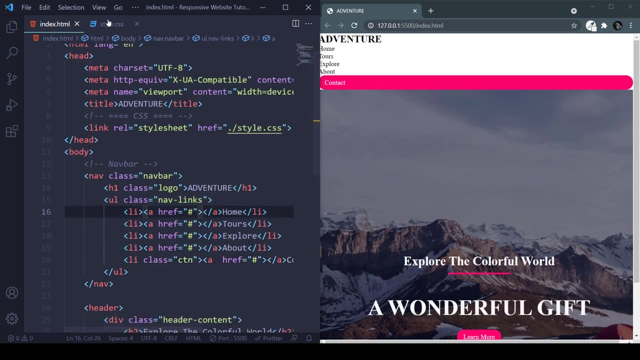 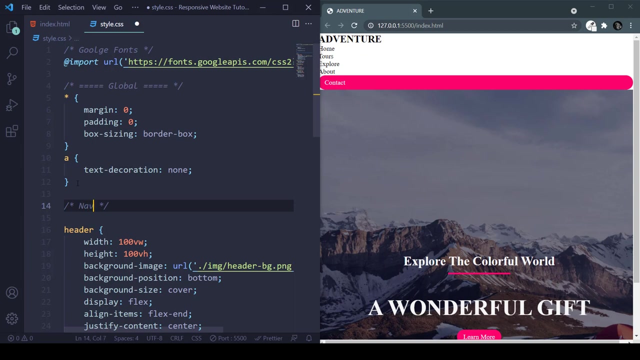 and i will add a class name of ctn to this and this is for our contact. add this class name to our ally. okay, now let's open our css file, get here, let's style our navbar, target our navbar and for this add display, flex and position. 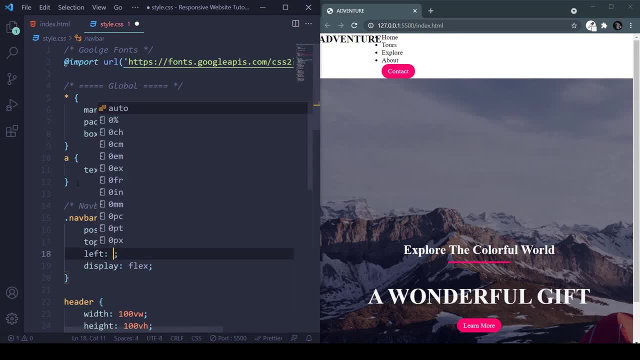 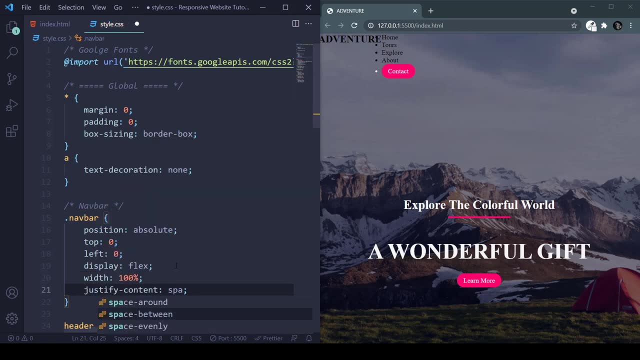 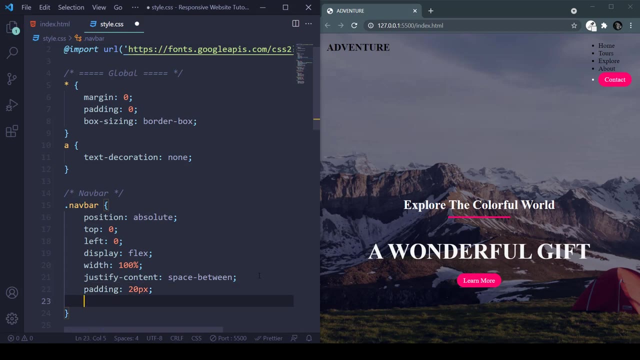 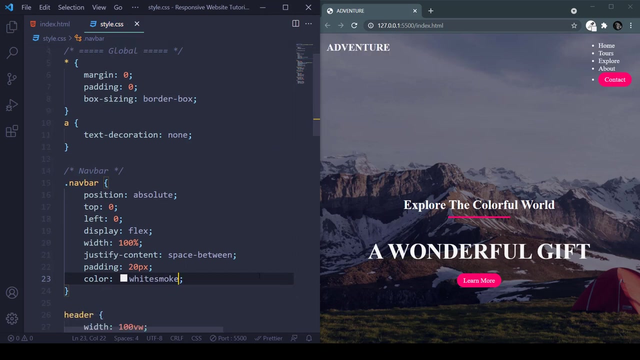 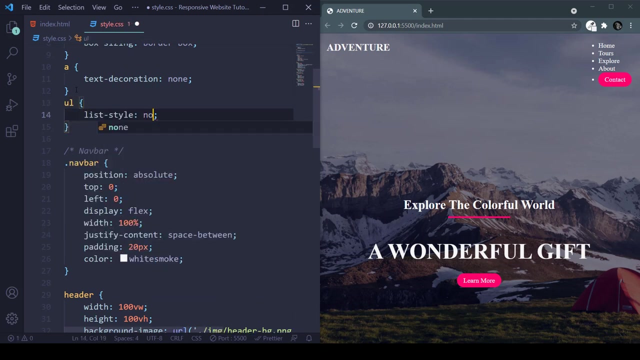 absolute and top 0 and left 0, and add width 100 percent and justify content space between and add a padding of 20 pixel and color and white smoke. right here, let's target our ul for this add list style. right here, let's target our nav links. 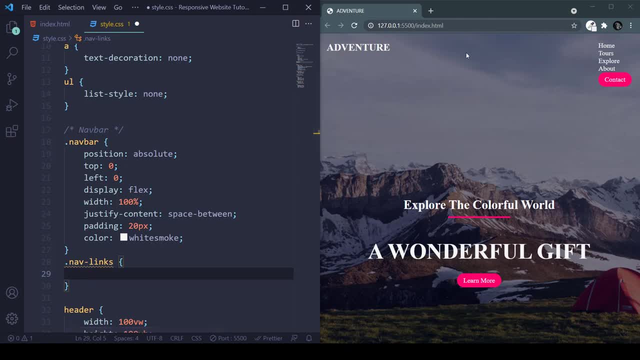 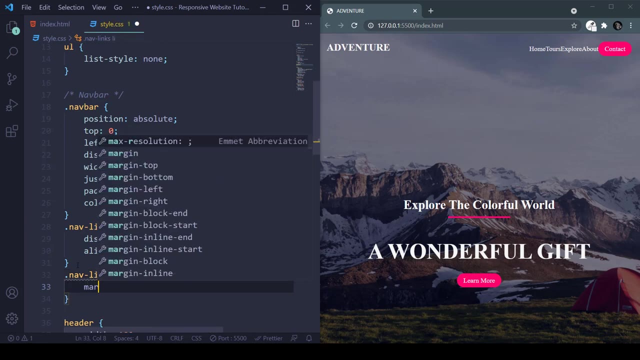 you can see, our nav links are aligned vertically so to make it in a horizontal. add display, flex and align items center and inside our nav links. target our ally for this: add margin, top and bottom zero and left and right 30 pixel. now you can see our beautiful navbar. 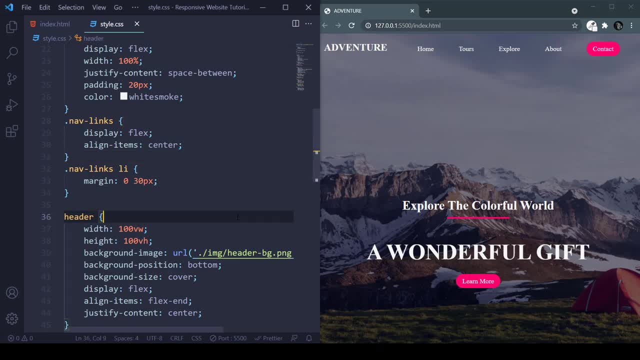 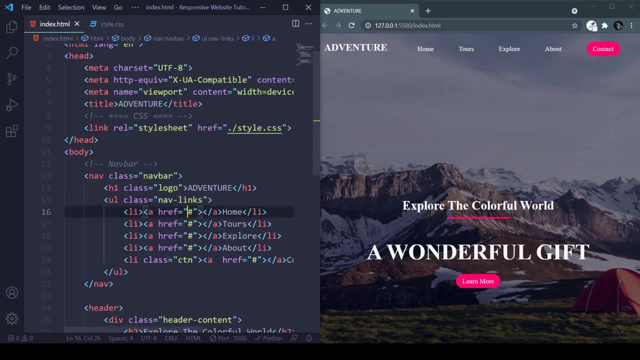 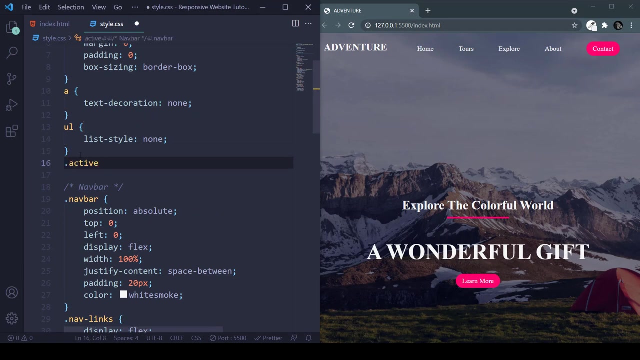 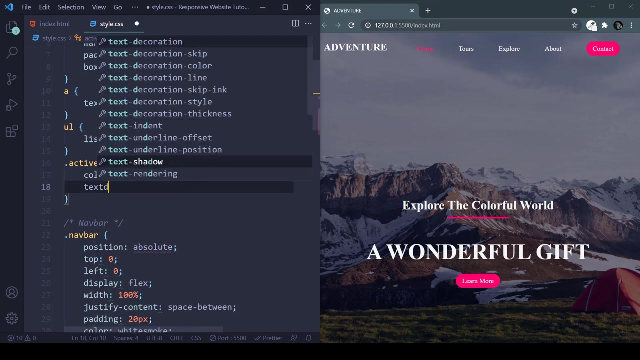 now let's make this responsive. so, to make this responsive, and before going to make it responsive, i will add a active class for this home. so inside our la, let's create a class here active, and inside our css file, let's target that active class and add color, this and add text decoration, underline and font weight: bold. 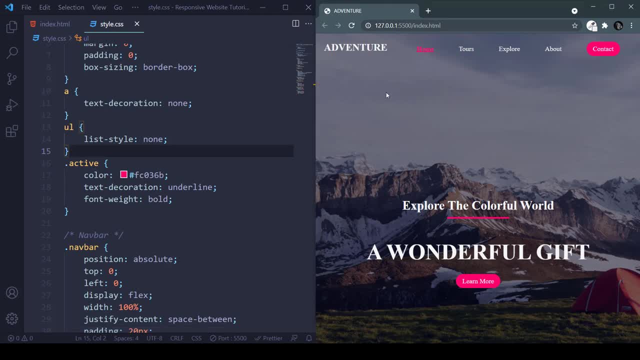 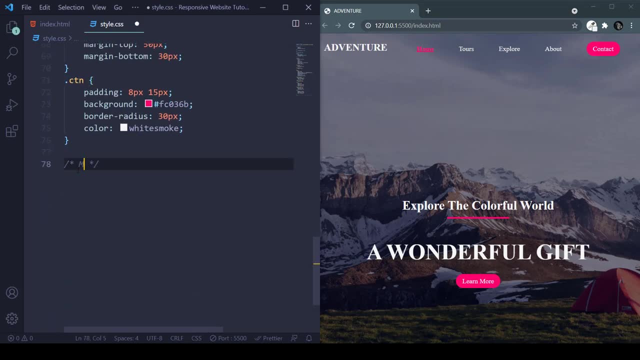 i can see our active class or active now link. have this color now. let's make this responsive. so to make this responsive at here, we will leave a comment of mobile device for this. add a media query: media only screen and max width of 850 pixel. target our now bar. 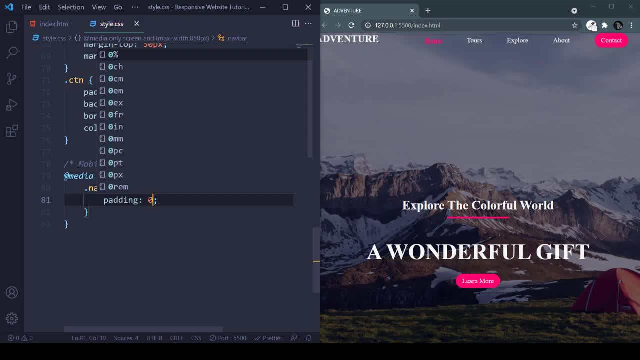 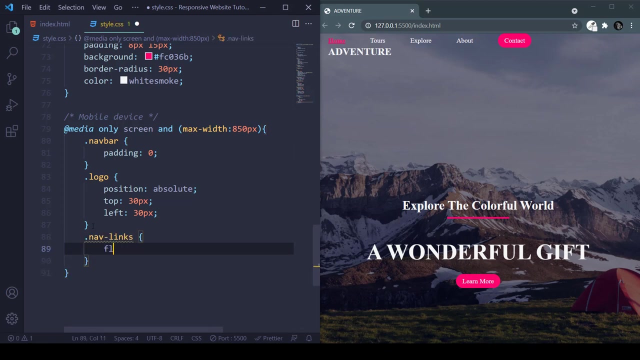 and make padding zero. after that, target our logo on this. add position absolute and top 30 pixel: left 30 pixel. you can see our logo here. now. let's target our now links. add flex direction column and width: 100 percent and height 100 vh. justify content center. now you can see our now links are here and inside our now links. 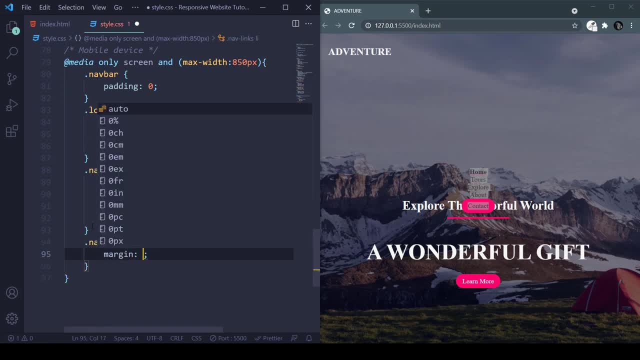 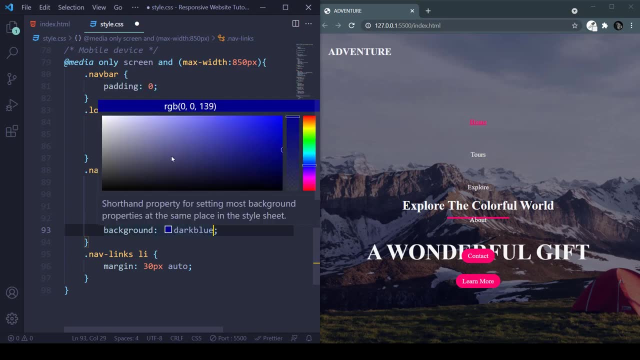 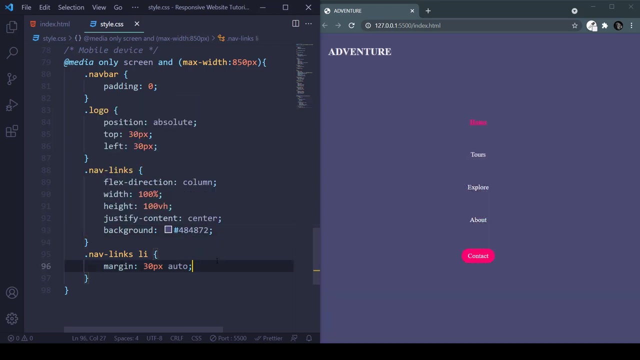 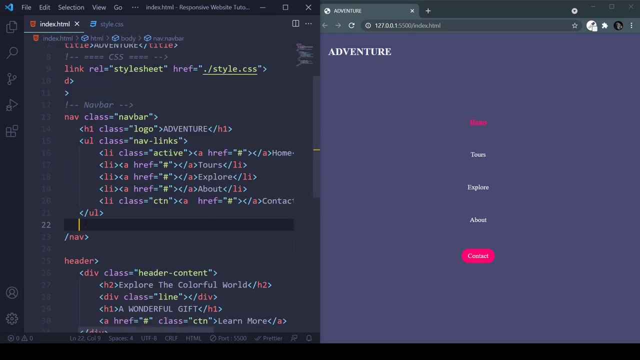 target our ally and add margin, top and bottom, 30 pixel and left and right auto. and for our now links, let's add a background of this color. now you can see our beautiful now bar here. now let's open our html file. inside our html file, after this ul, let's add a image with a class name of menu button. this will be inside our images. 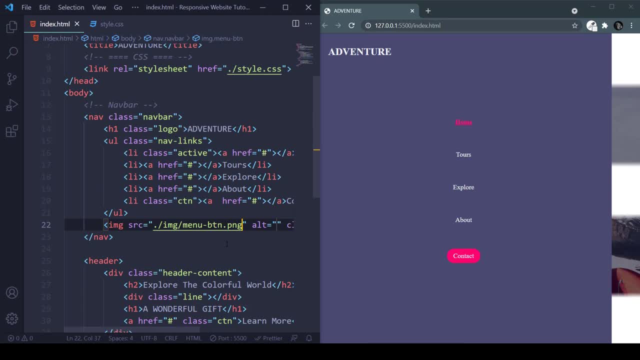 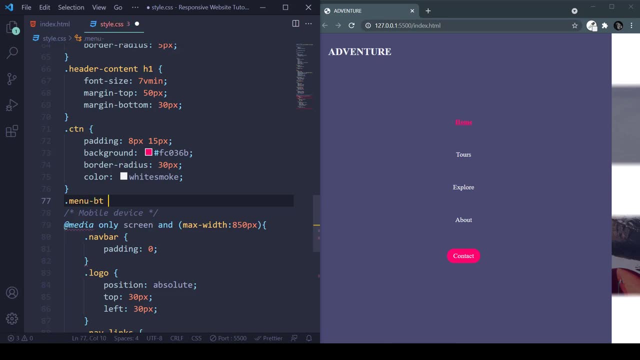 on menu button: dot png. now let's open our css file and target that menu button and add position: absolute and top 30 pixel and right 30 pixel. i can see our menu button here. now let's change this width to 40 pixel. awesome, and cursor pointer. and now, if we click on this menu button, our 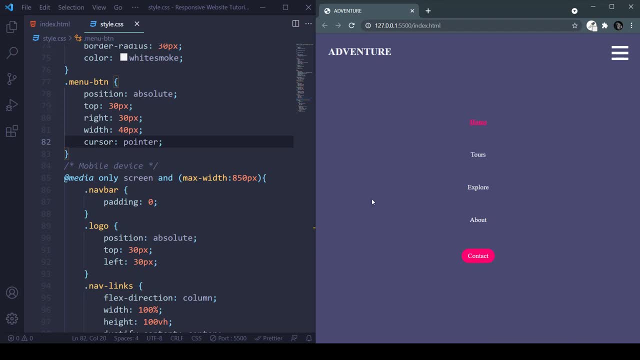 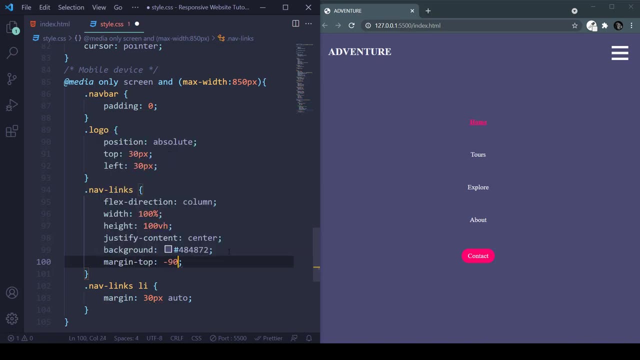 our mobile now have to appears and if i click again it has to disappear. and now if we click on this menu button, our our mobile now have to appears and if i click again it has to disappear. so to make that inside our now links, add margin top minus 900 pixel. 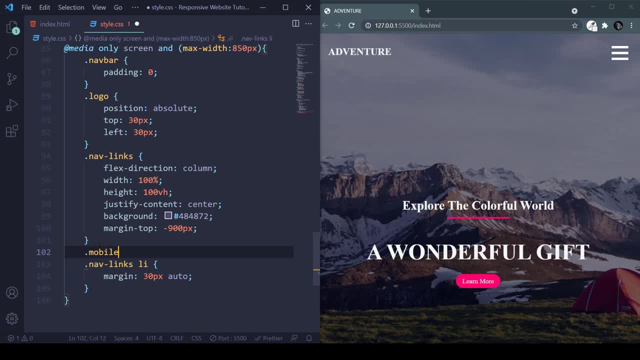 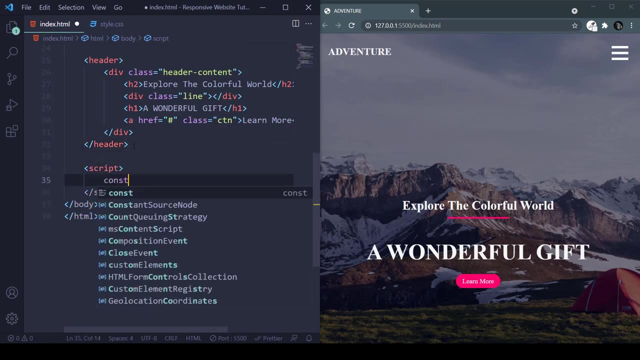 and add a class name here of mobile menu and add margin top 0 pixel. now open our html file and before this body tag let's add a script tag and inside this let's get our our menu button- document dot, query selector and menu button and get our now links. 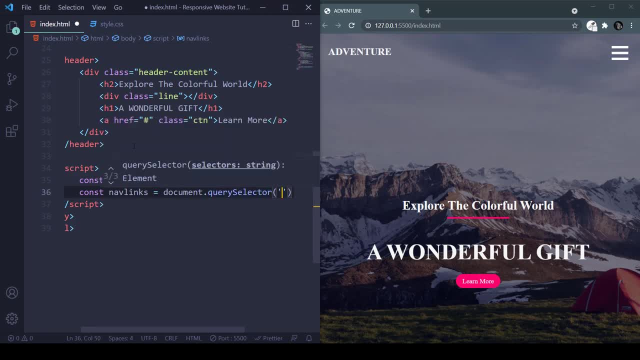 document dot query selector. now links. next. you need to add this dot here. document dot query selector: 額 key. These Questo now links next. you need to this next here and now links next nextfor a lot of things is coming out. let's first start writing some of these internet options: documentquerydcom- lot business aims like uh network countriesawputcom. now linksраст will worry you with. now anything belongs to your service: us tips, etcruct pursued through the linux시간, credithöbe and representacom connection to normalization, which previses also should not be addressed in this section. say, a tutorial for past 2 went through other parts, so just keep online benefits etc. gemstone contact recipes. 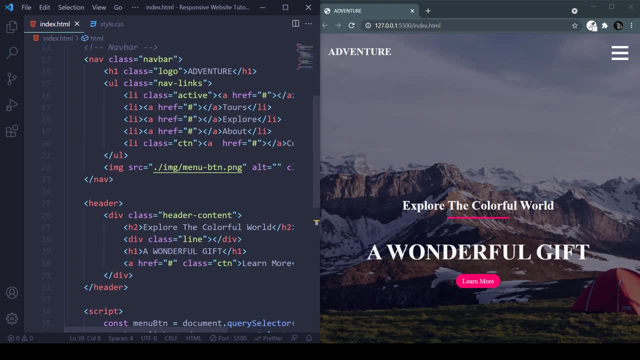 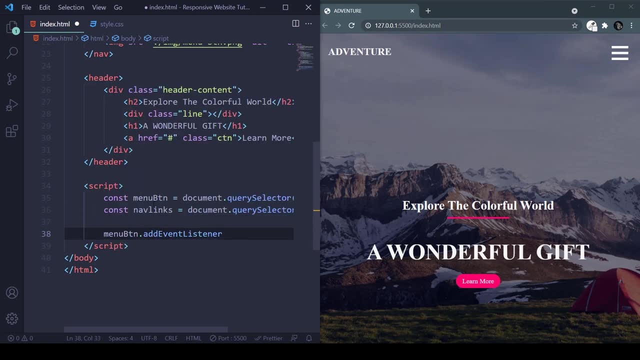 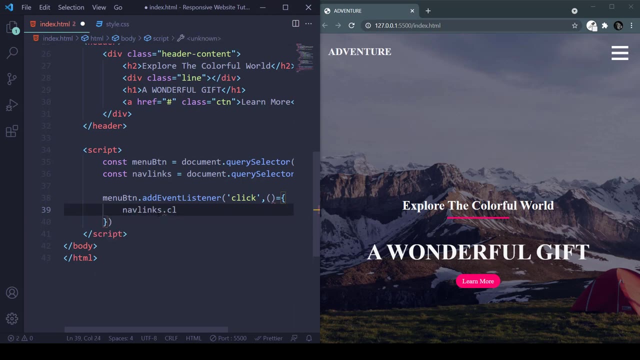 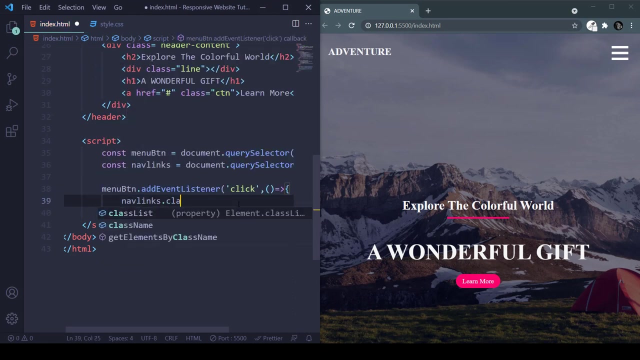 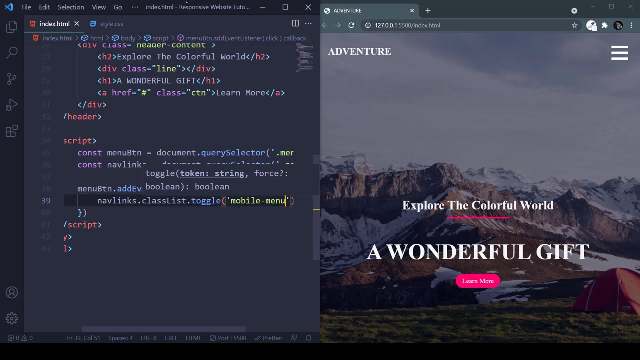 to add this dot here and the exact name as we given here and now for our menu button. let's add a event listener on click for our nav link. add a class list nav links dot. class list- dot. toggle that mobile menu now if I click on this menu. 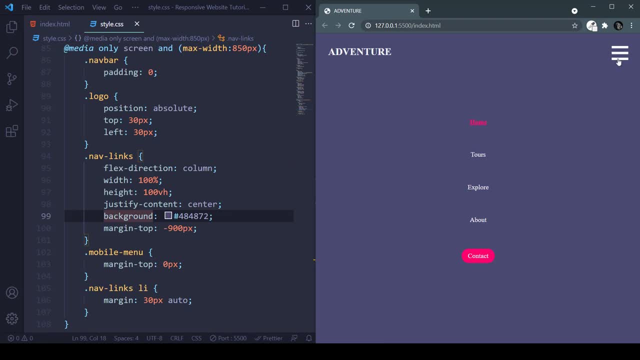 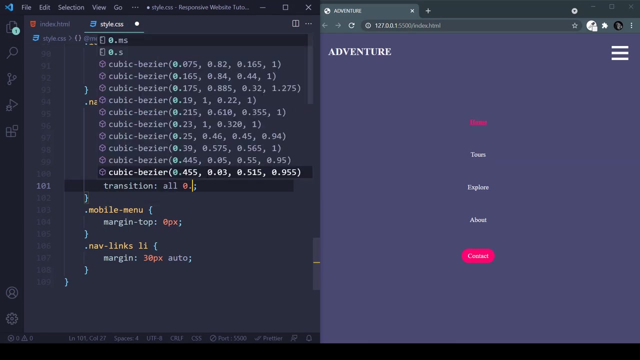 button on mobile menu appears and I feel, and if I click again, it disappears. now we have to add a smooth animation for this, to add that inside our nav links, a transition on 0.5 seconds is: if I click here, our mobile menu appears from the top and for 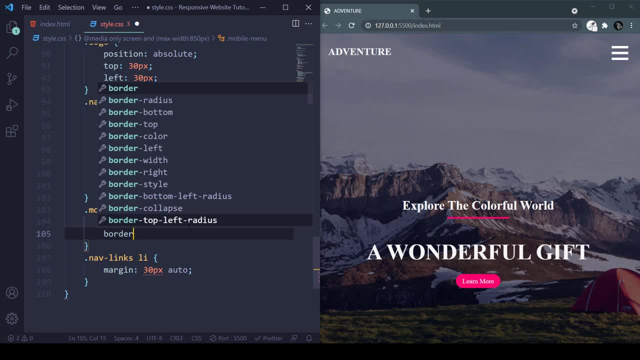 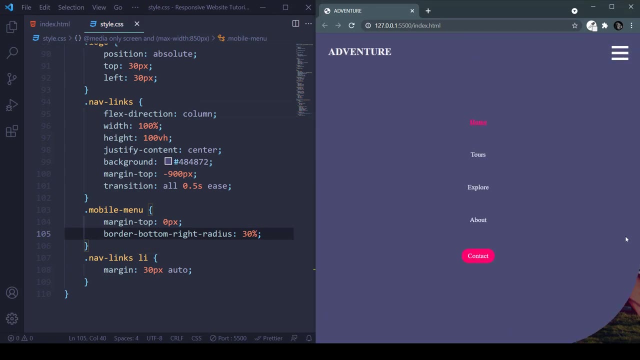 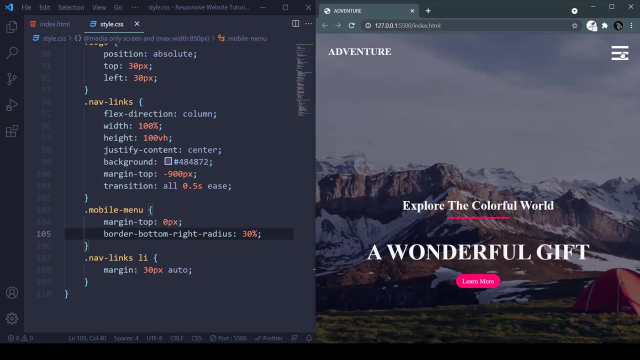 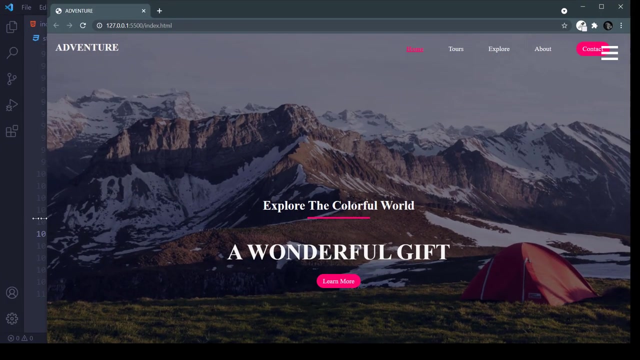 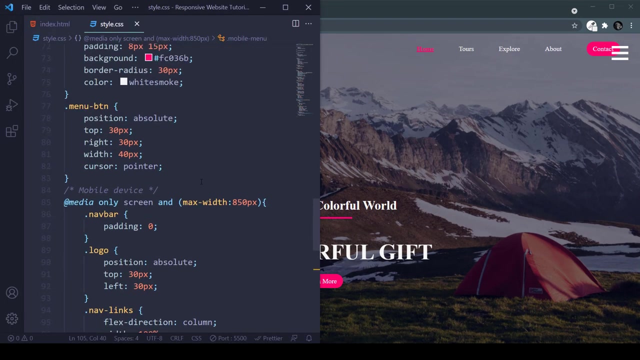 our mobile menu. add border bottom right radius and this 30%. I can see this beautiful border radius here. if we click here disappears and if and if we click again it appears. now our beautiful responsive now bar is completed and you can see our mobile menu is appearing here. we have to remove that for our mobile menu. add display none. 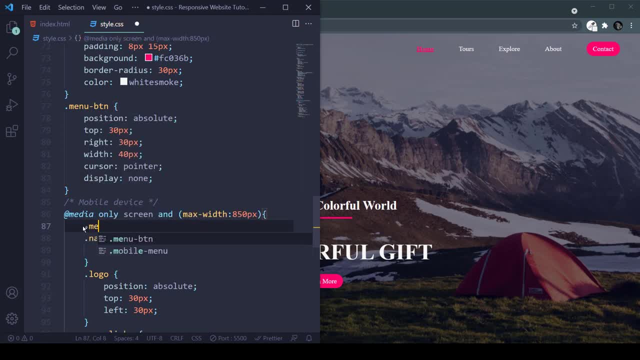 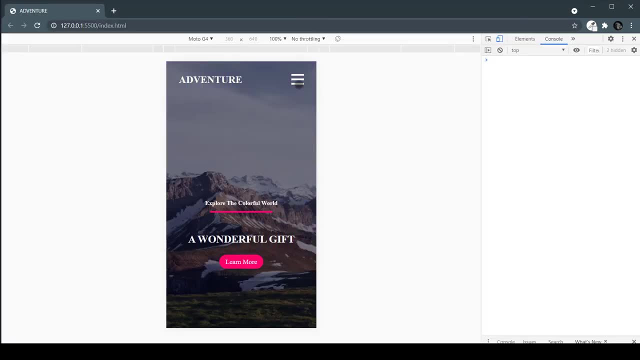 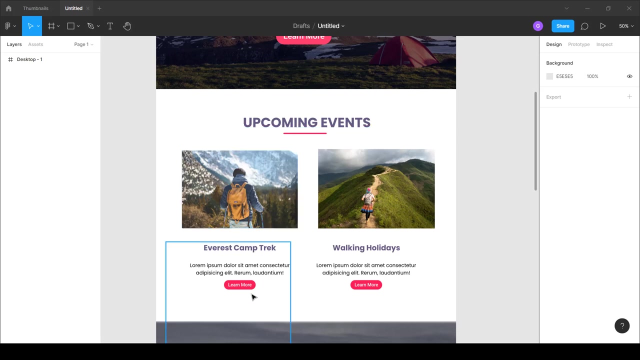 and inside our mobile screen, target our menu button and add display block. awesome, I can see our beautiful responsive header section. full screen header section. and now what is completed? now let's move on to our next section, which is this: events. so let's open our HTML file and, after our 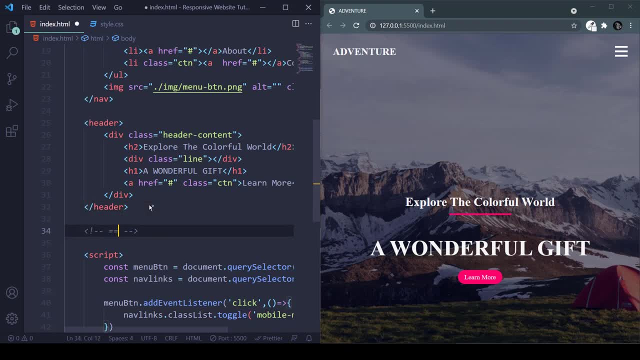 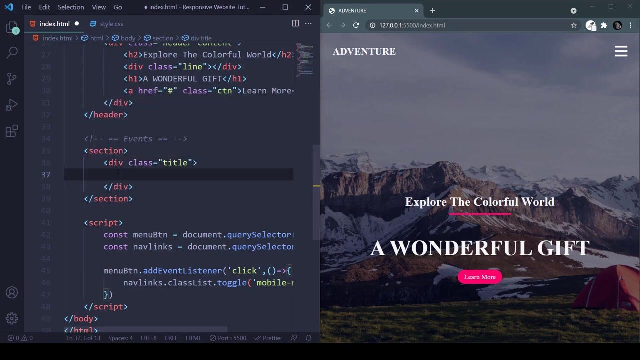 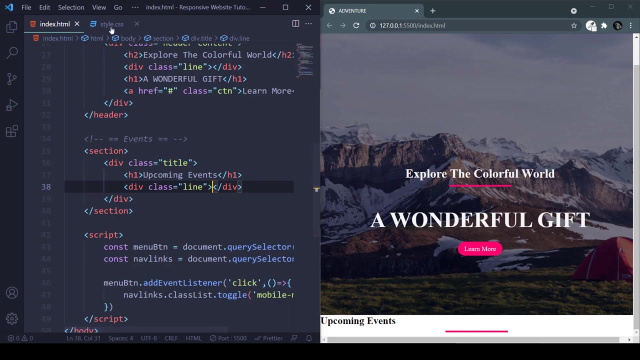 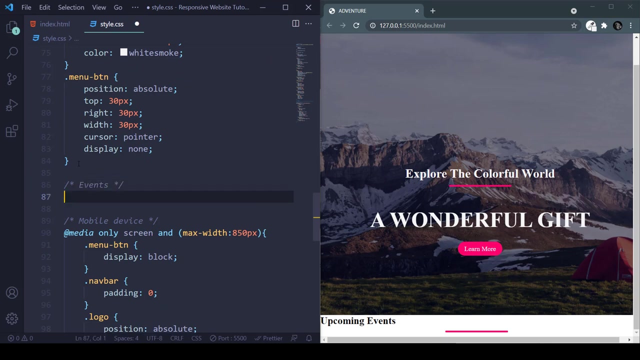 header section, I will create a section called events section, with a class name of events. I will create a section and inside that we have our title. inside our title we have a h1 with a text upcoming events and a line, and inside our CSS file, let's, let's target that, let's target our section and 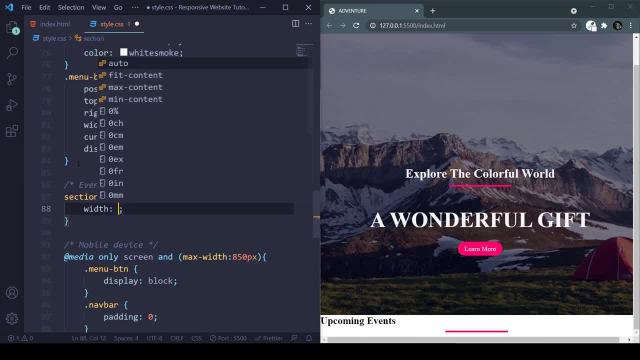 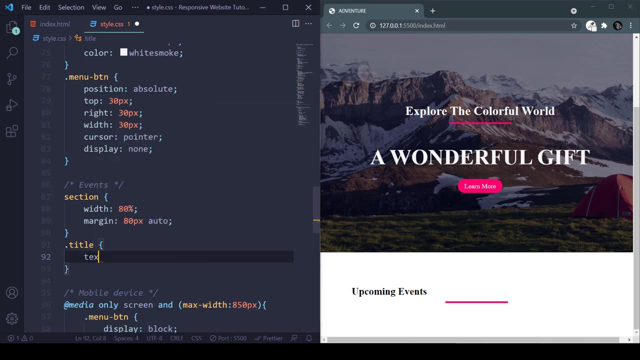 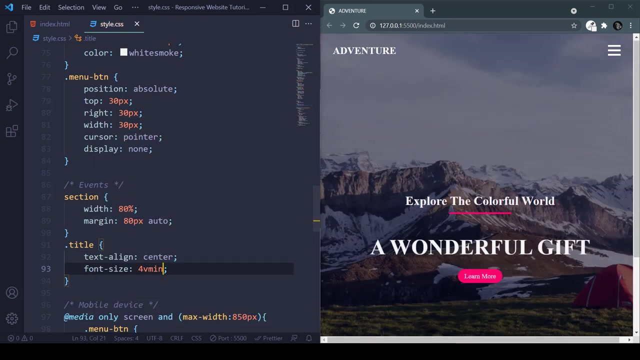 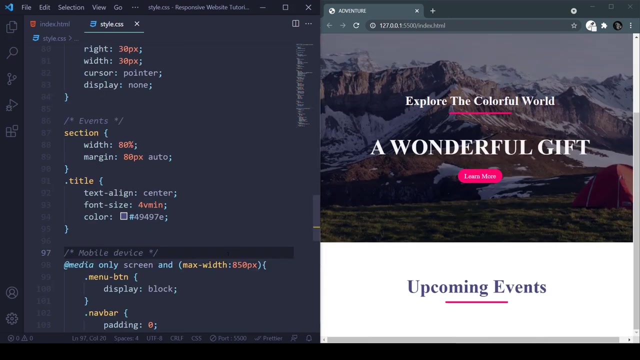 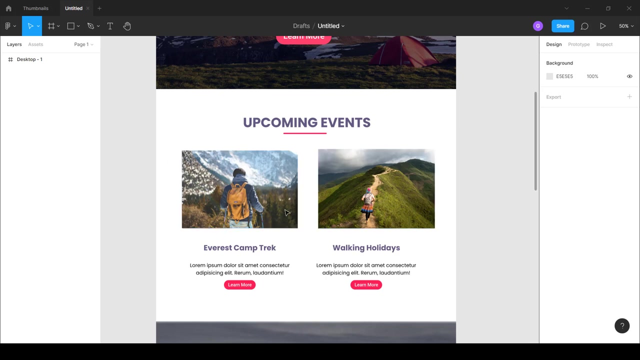 for this. add a width, 80% and margin, top and bottom, 80 pixel and left and right auto. let's target our title for this, add text, a line center and font size for women and change color to this color and after this title, let's add these images: if you can see this easier, row and inside this: 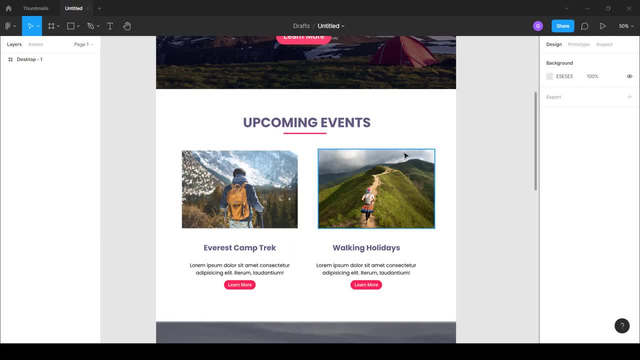 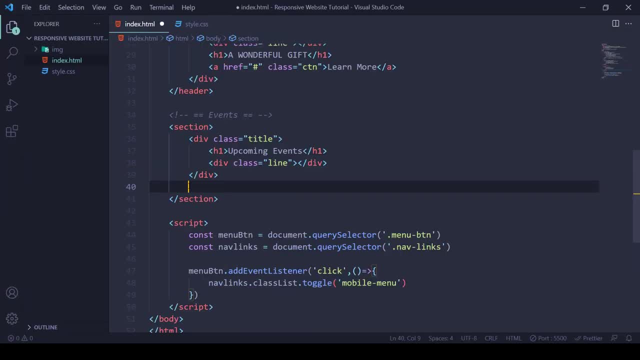 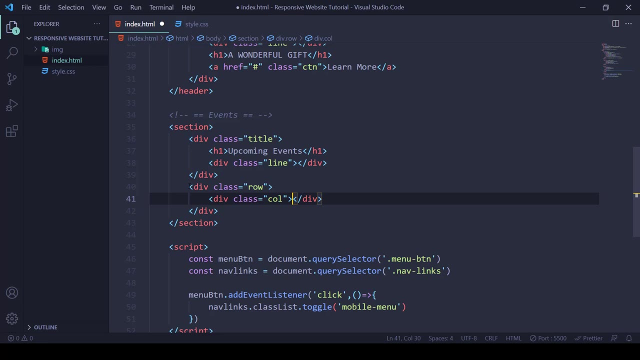 row we have two columns: which is for this image and this text, and for this image and this text. so inside our HTML file, after the title, I will create a row. inside that we have a column. inside that column we have a image, which is our image inside. 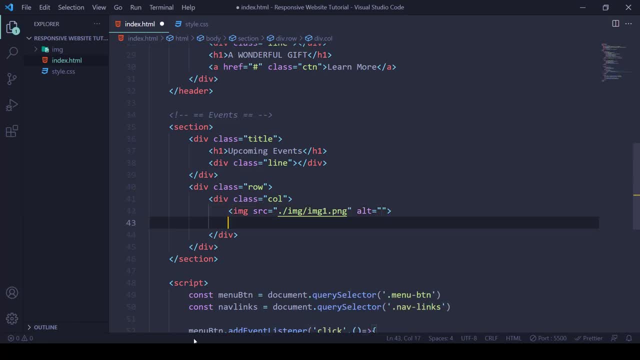 our images, or image one, and after that we have this h2 and this text and your learn more button. create a h4 you called EverestCampTrick, and after that we have a p tag with some dummy text and a anchor tag with the class name of ctn with the text learn more and 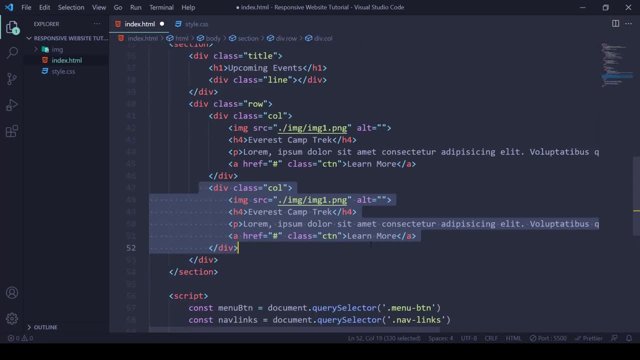 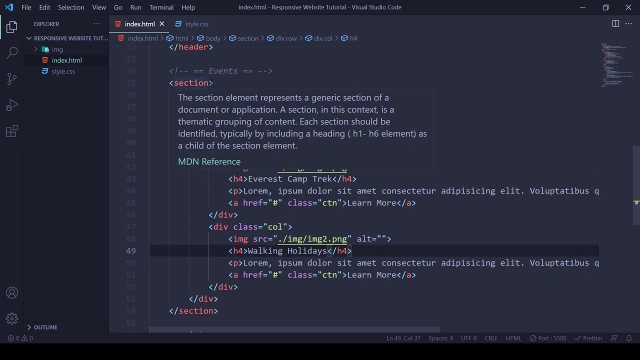 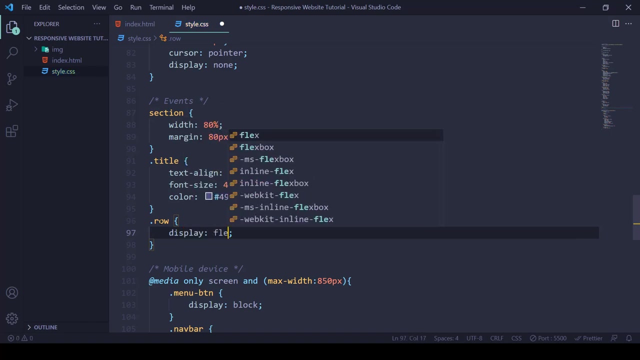 duplicate this column and add here: add image to and change this title to walking holidays and for the section add a class name- events- and add here target overflow and for this add display flex. I can see these images here and allen items st now inside our raw. 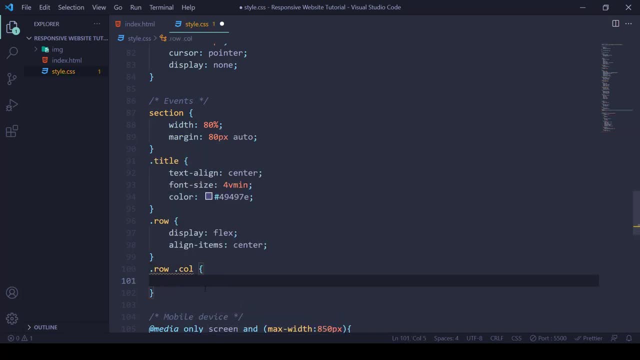 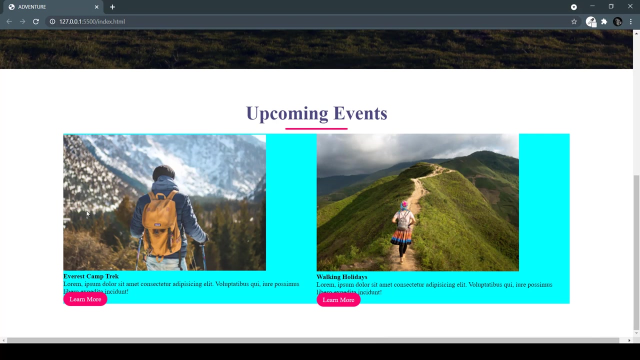 absoluter column. for this, add a width of 80%. said our column, target or image, and for that animation of 80% and our row, add a width of 100% and justify content space between. to see what's happening there, let's add a background for this dark blue. you can see our image, one of. 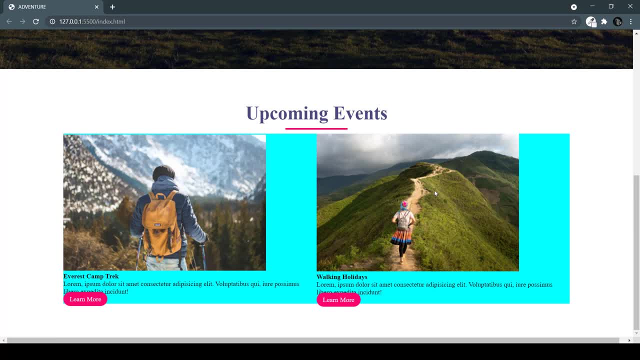 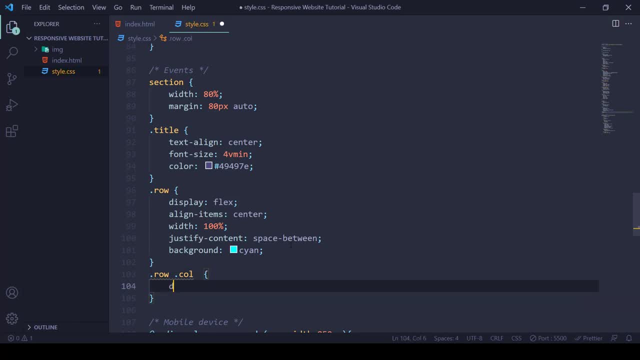 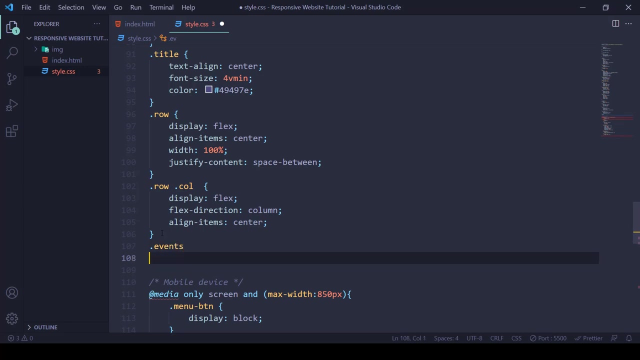 the image in it is a starting of this flex and this image is at here to make this, to make this go all the way up here inside our column and display: flex and flex direction column and align items Center. you can see these are perfectly aligned. now let's remove this background color now inside our events target, our 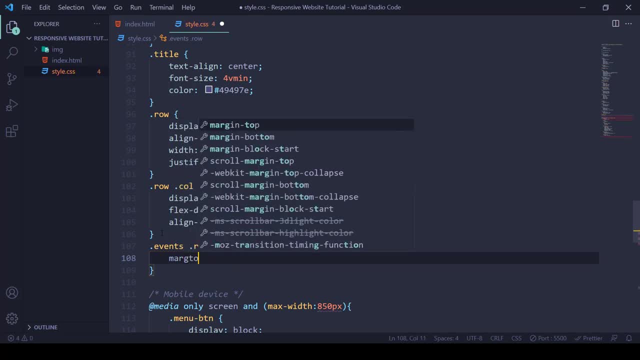 row and for this add margin top 50 pixel. I added- I didn't add in margin top for this row here because I want to reuse this into another sections, so I did even I targeted this events and added margin top 50 pixel here for our hits, for let's. 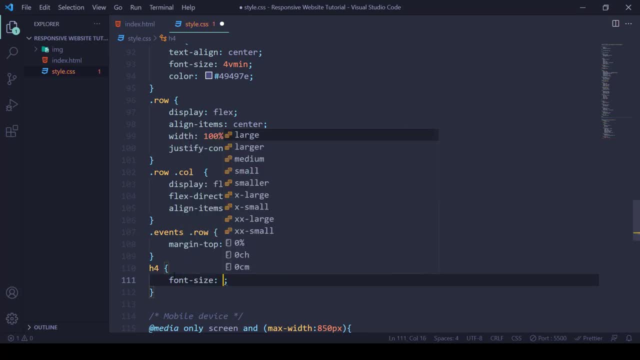 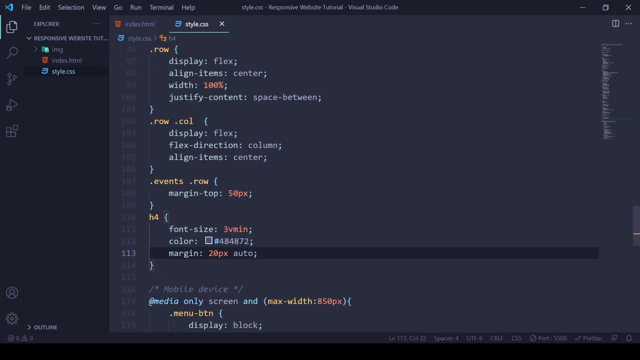 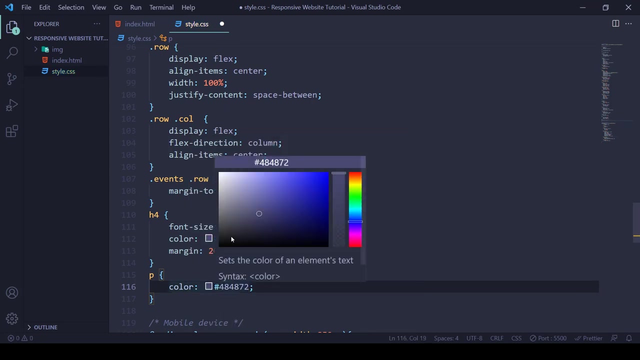 add a font size of three women and color of this color and add margin top and bottom on the pixel and left and right auto to add color will total one of the two. let's try target or p-top at this. add a color of this and add padding 0 pixel. 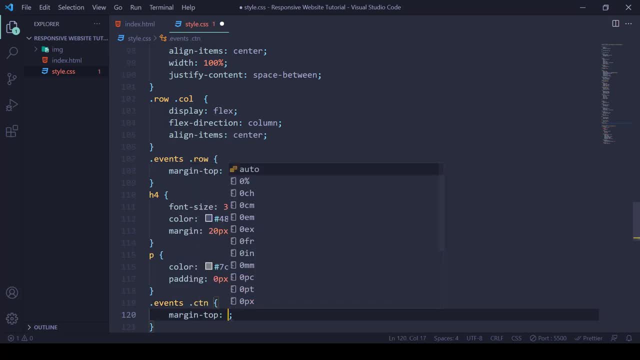 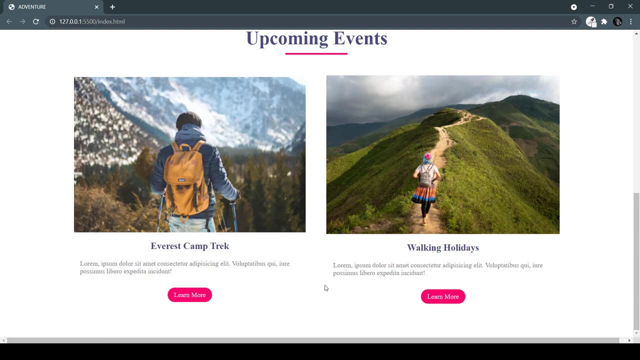 top and bottom and left and right for the picture, and inside our events. a BRT Series of elements will be located in this table. now, getting to our color, I will select. see our event section is beautiful and completed and now you can see there is a horizontal. 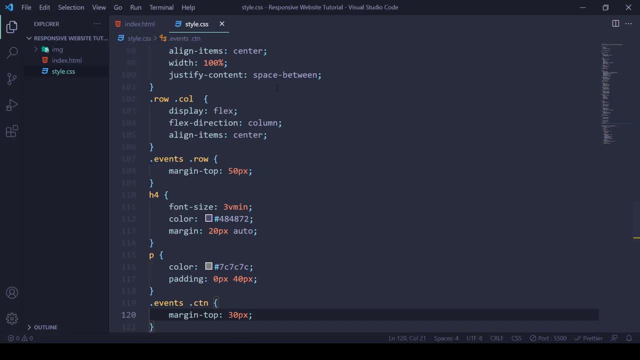 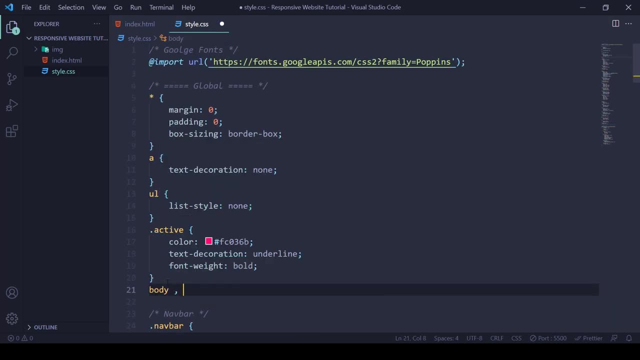 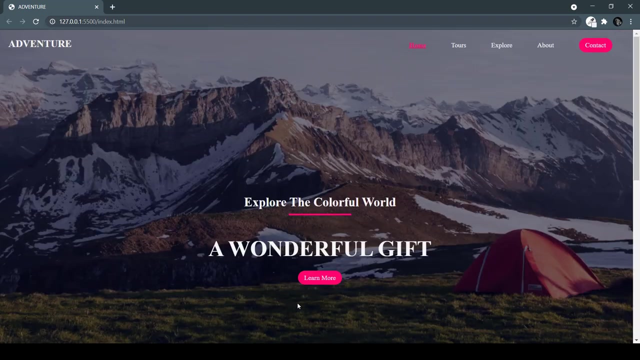 scrolling here to remove that. inside, open our css file and inside this let's target our body and html. for this: add overflow x hidden. you can see there is no horizontal scrolling here. now let's move on to our next section. we'll create a section with the class name of explore. 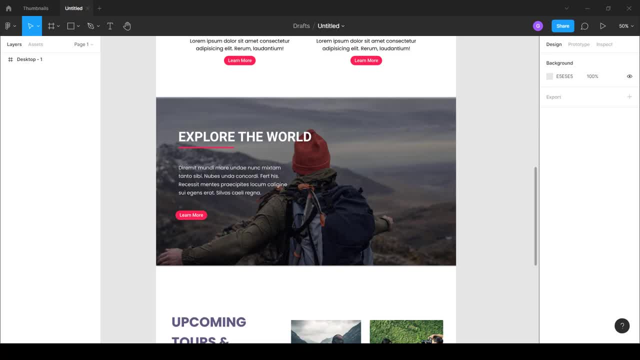 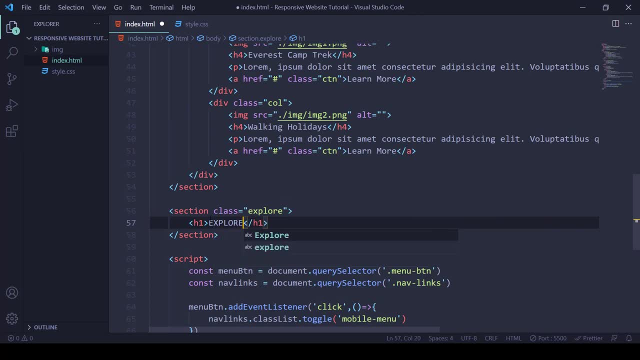 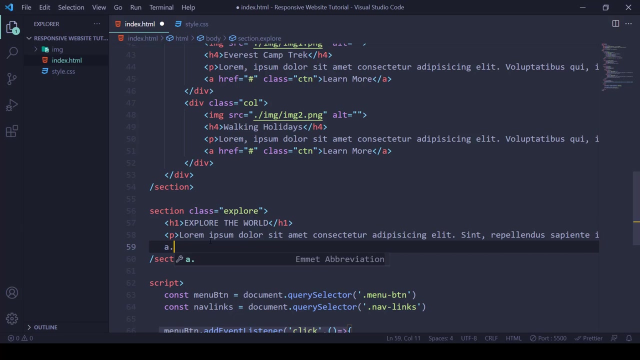 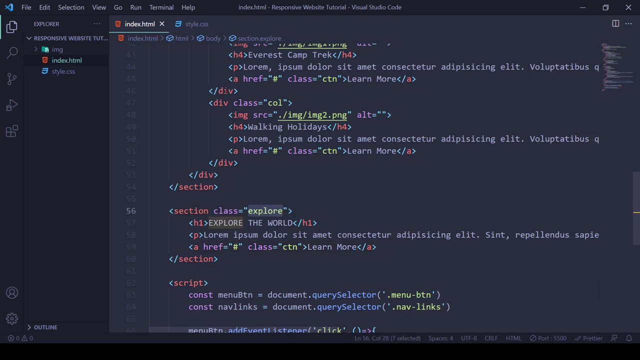 inside this we have a h1 with the text explore the world, and after that we have a p1 tag with some dummy text and after that we have a anchor tag with a class m of ctn. this will be our learn more button. now let's target this explore inside our css file. 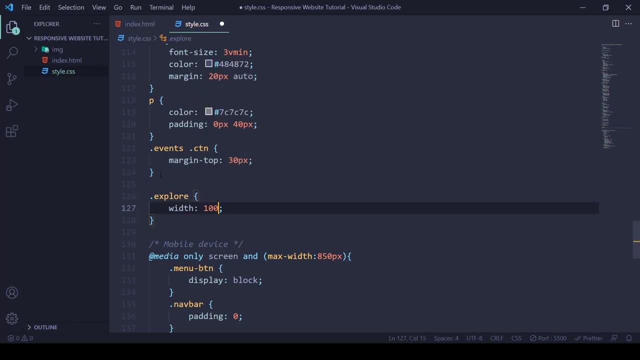 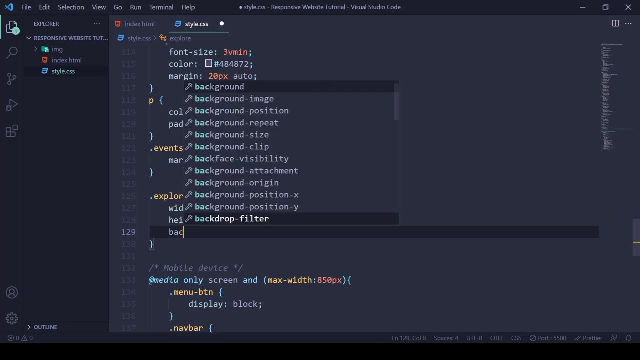 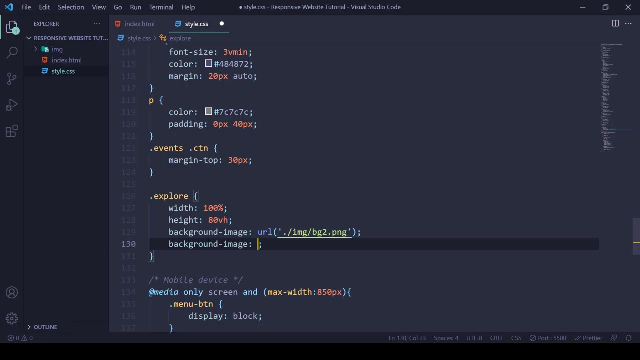 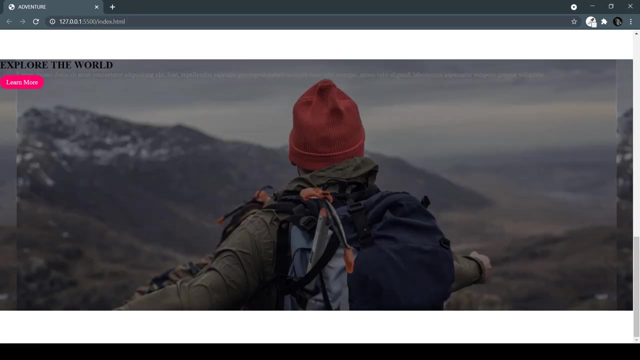 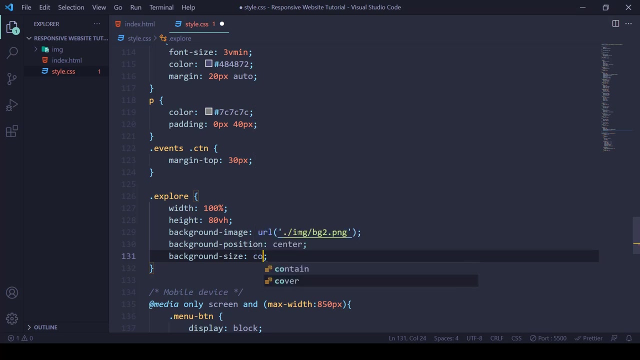 for this, add a width of 100 percent and a height of 80 bh and add background image. this will be url and inside our images: bg2.png. you can see this image here. for this: background position center and background size, cover and background. repeat, no repeat. 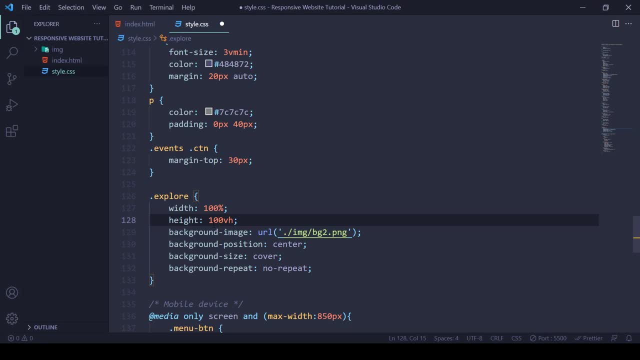 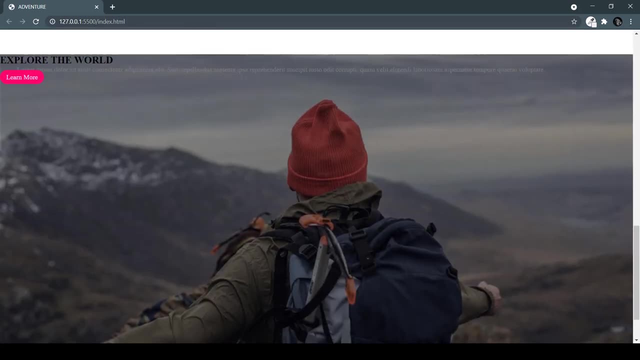 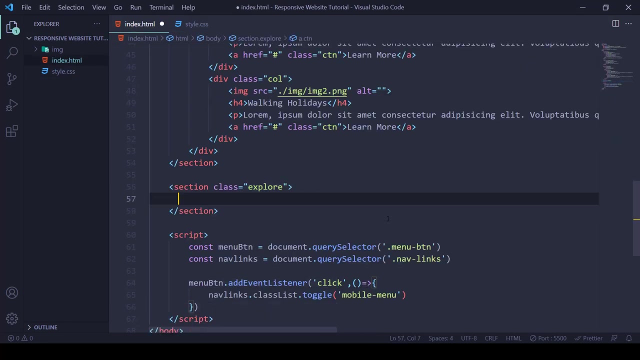 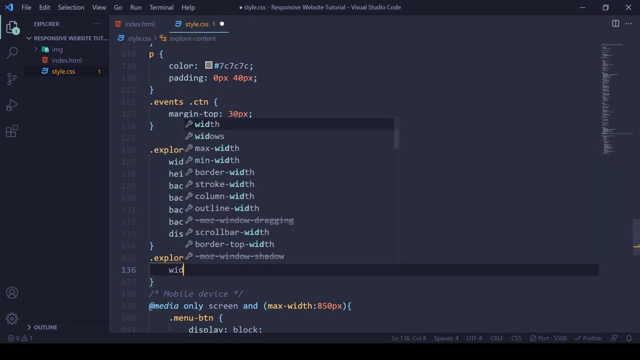 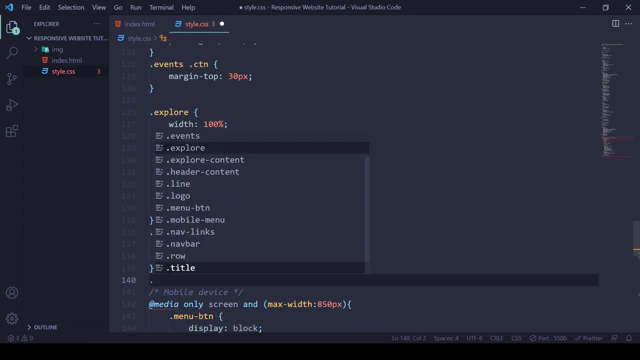 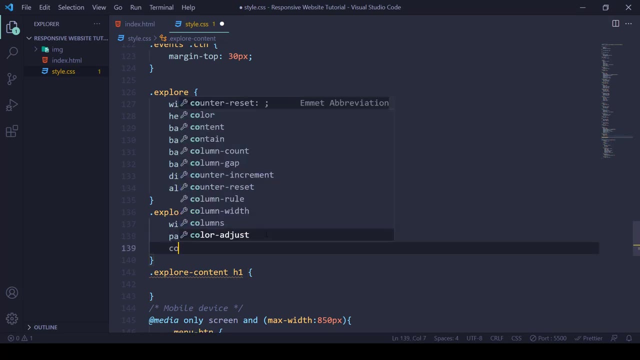 for our explore align items center, for our explore align items center, for our explore align items center, inside our explore content, inside our explore content, inside our explore content, target, our h1. and for all of these, let's add a color of, and for all of these, let's add a color of. 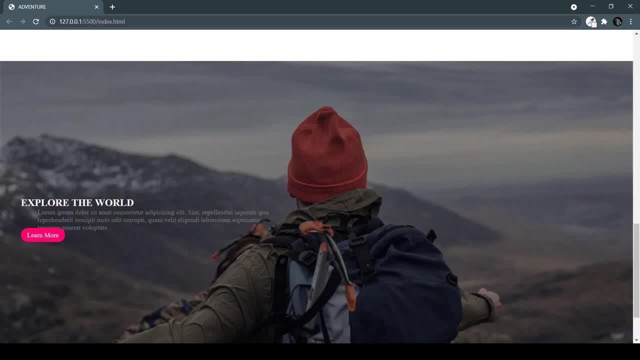 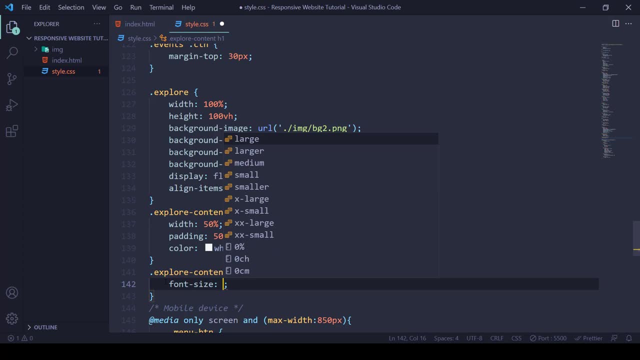 and for all of these, let's add a color of white smoke. now for our h1. add font size. now for our h1. add font size. now for our h1. add font size of seven beaming margin: bottom of seven beaming margin- bottom of seven beaming margin: bottom 50 pixels and makes this with to 60. 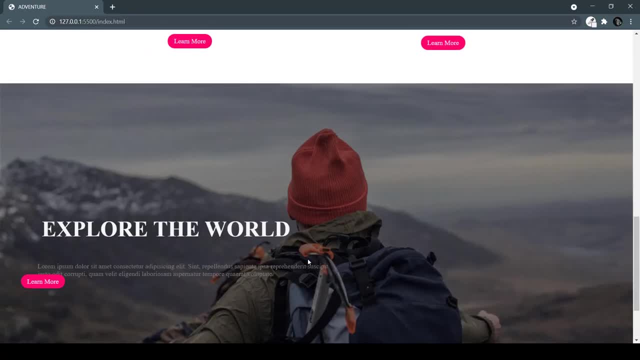 50 pixels and makes this with to 60: 50 pixels and makes this with to 60 percent, percent, percent. this would. this will be nice. i guess this would. this will be nice. i guess this would. this will be nice. i guess awesome. now inside our explore content. 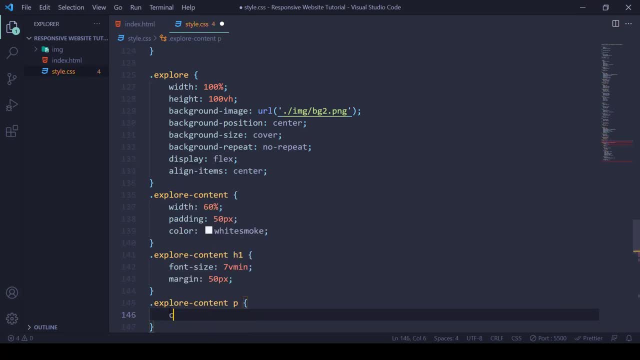 awesome now inside our explore content. awesome now inside our explore content target, our p tag target, our p tag target, our p tag for this: add a color of white to something like this. of white to something like this, of white to something like this, so this will be visible. 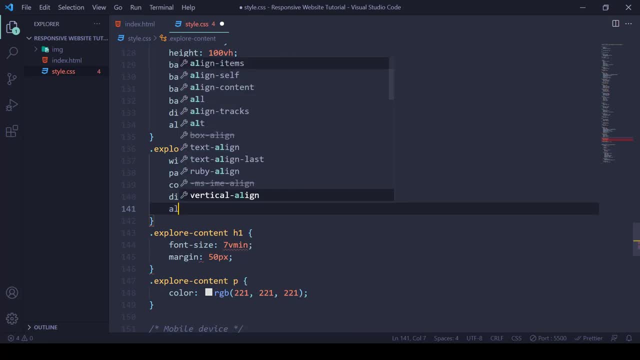 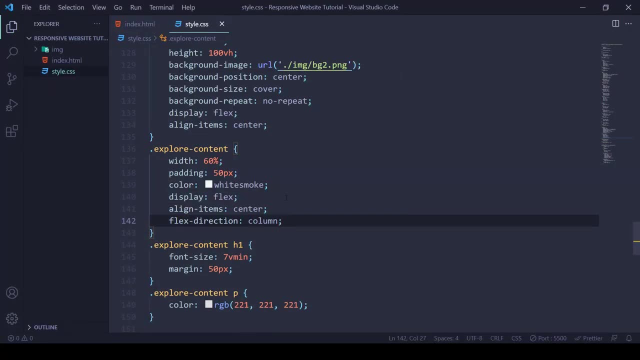 so this will be visible. so this will be visible for this. add display flex for this. add display flex for this. add display flex. then items, then items. then items: center, center, center influx direction column and inside our influx direction column and inside our influx direction column and inside our explore content, target our ctn and add. 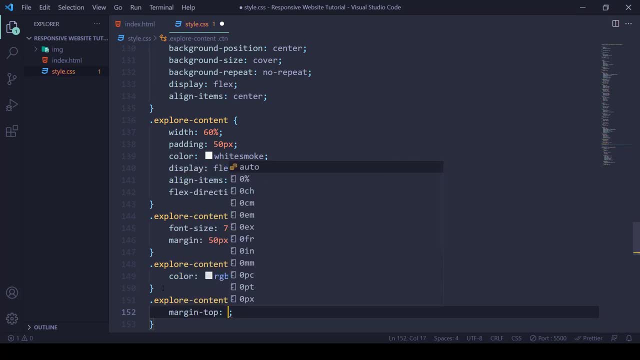 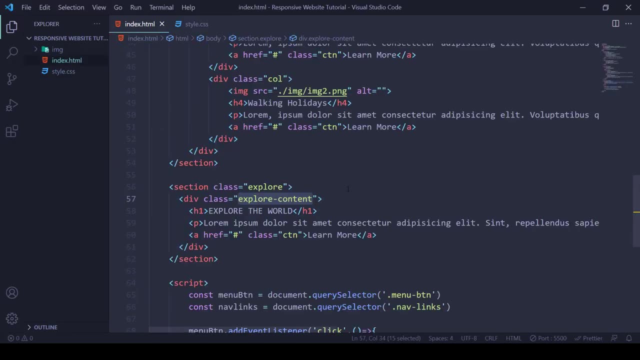 explore content: target our ctn and add: explore content- target our ctn and add margin top 40 pixel. awesome now let's margin top 40 pixel. awesome now let's margin top 40 pixel. awesome now. let's open our HTML file and after this, h1. 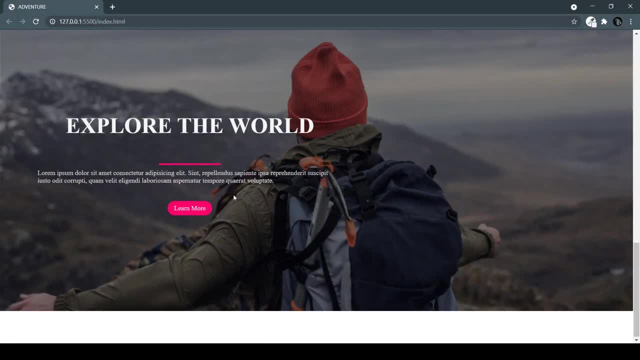 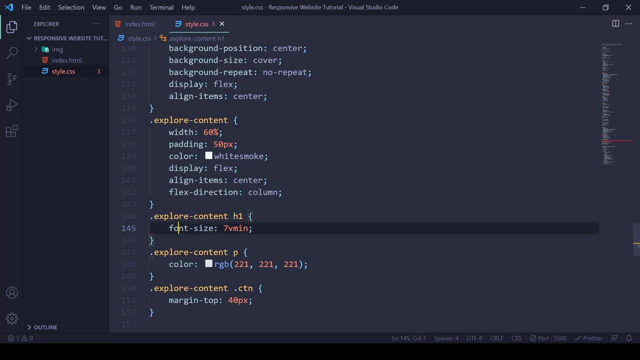 open our HTML file and after this h1, open our HTML file and after this h1, let's add a line. and now let's move this. let's add a line, and now let's move this. let's add a line, and now let's move this margin here and inside our explore. 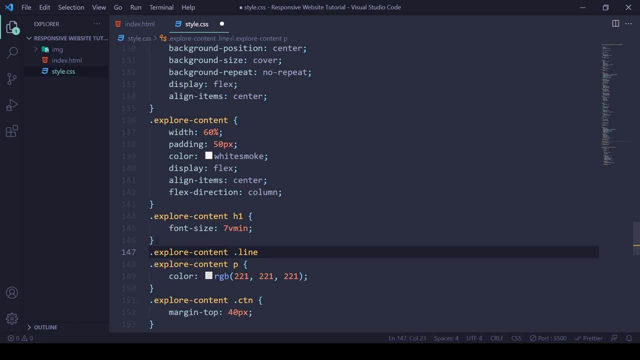 margin here and inside our explore margin here and inside our explore content target- our line for this and the content target our line for this and the content target our line for this. and the margin margin: bottom: 50 pixel you can. margin margin: bottom: 50 pixel you can. 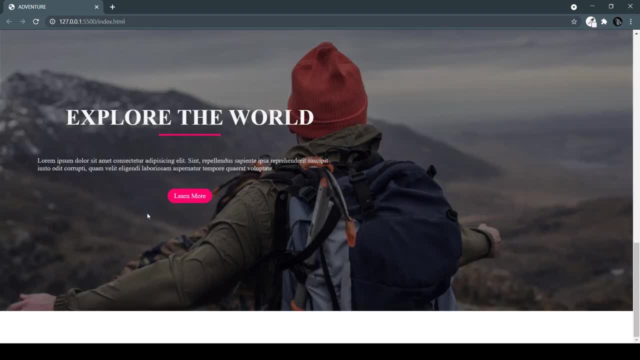 margin: margin bottom: 50 pixel. you can see our beautiful background image with. see our beautiful background image with. see our beautiful background image with this beautiful text. and now let's move this beautiful text. and now let's move this beautiful text. and now let's move on to our next section, which is this: 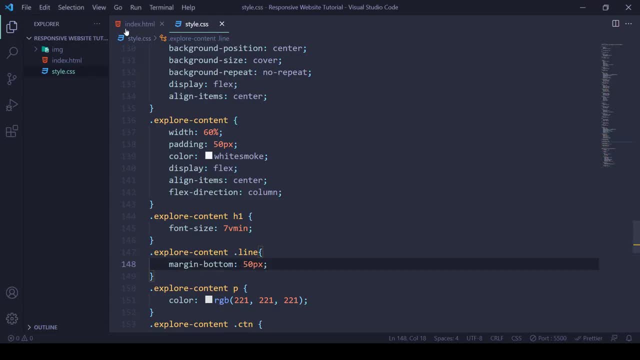 on to our next section, which is this. on to our next section, which is this: coming tools. so now let's open up coming tools. so now let's open up coming tools. so now let's open up our HTML file. and after this section, we our HTML file, and after this section, we. 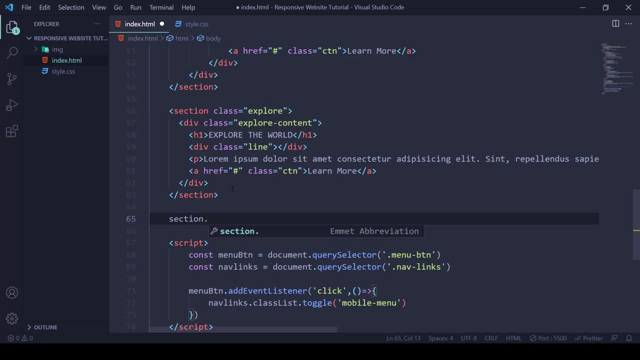 our HTML file and after this section, we will create another section with a class, will create another section with a class, will create another section with a class name of tours. for this I will add a row name of tours. for this I will add a row name of tours. for this I will add a row and inside that we have a column inside. 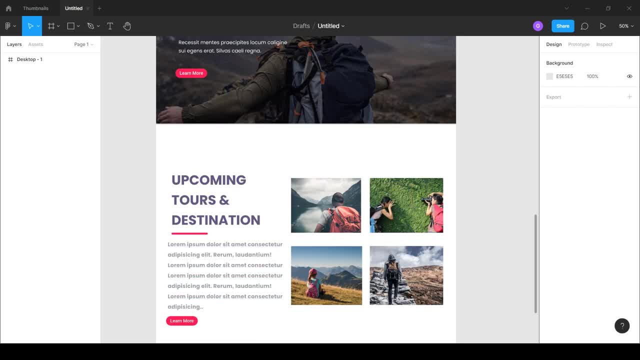 and inside that we have a column. inside and inside that we have a column, inside this first column. we have this. it's one, this first column. we have this. it's one, this first column. we have this. it's one text and this paragraph. so I will create. 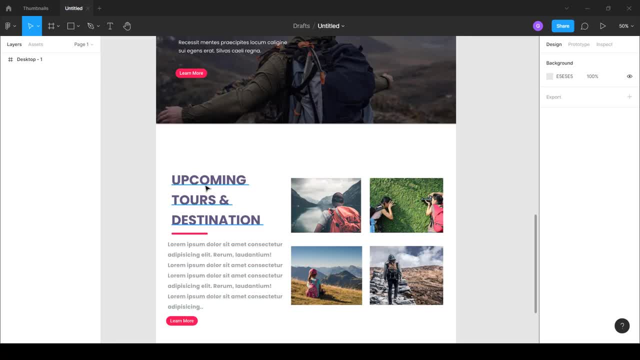 text and this paragraph. so I will create text and this paragraph. so I will create a h1 with this text. after that, we have a a h1 with this text. after that we have a a h1 with this text. after that we have a p-tank with some dummy text and after 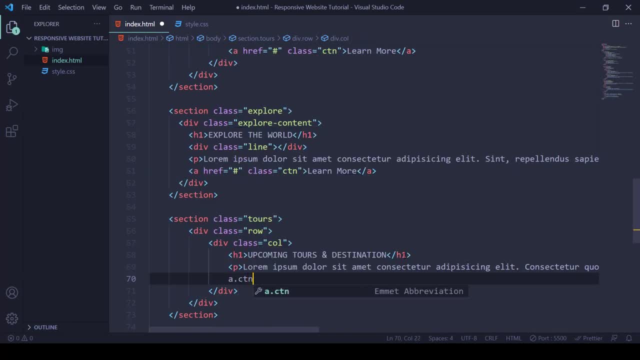 p-tank with some dummy text and after p-tank with some dummy text and after that we have- we have our anchor tag: the that we have. we have our anchor tag: the that we have. we have our anchor tag: the classroom of CTN and this will be learn. 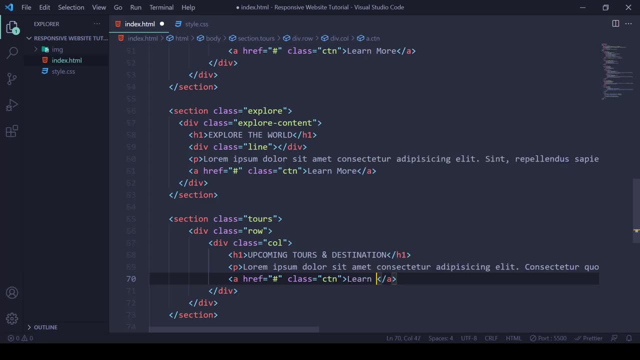 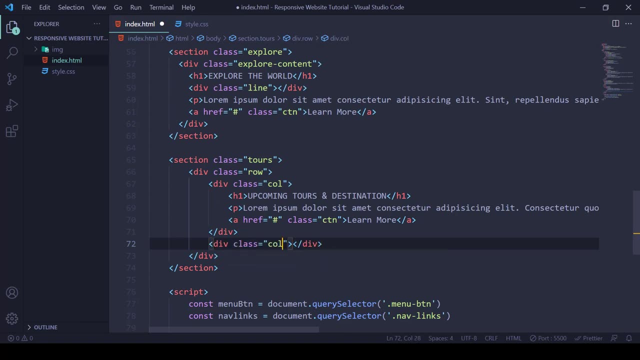 classroom of CTN, and this will be learn classroom of CTN, and this will be learn more button. now. let's add another more button. now. let's add another more button. now let's add another column and add a class name for this column and add a class name for this. 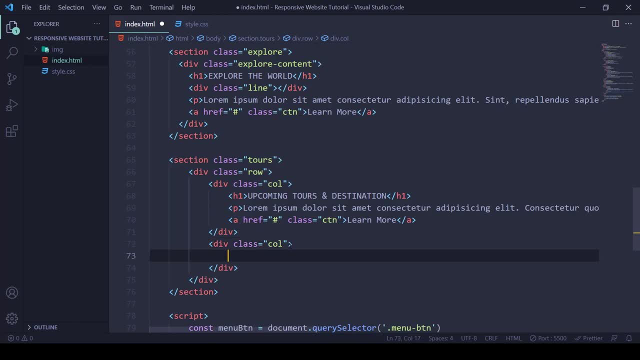 column and add a class name for this and add a class name off and insert this. and add a class name off and insert this. and add a class name off and insert this column. let's add a do called image column. let's add a do called image. 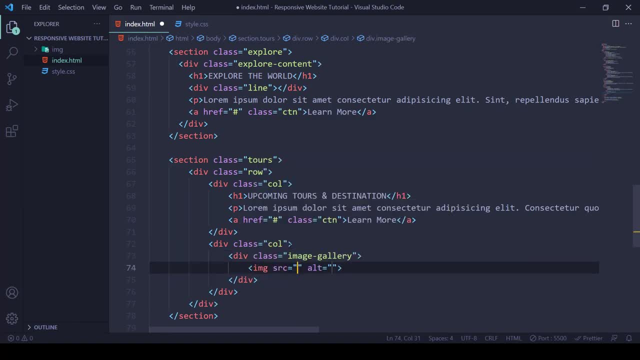 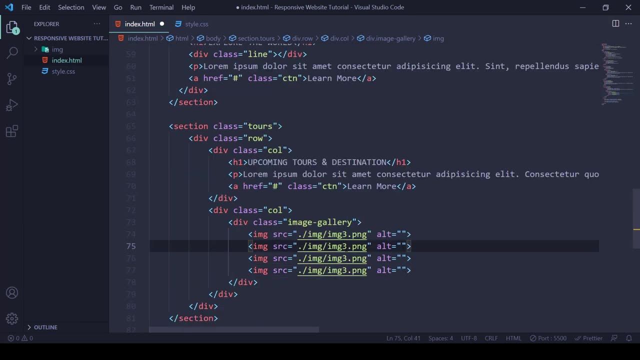 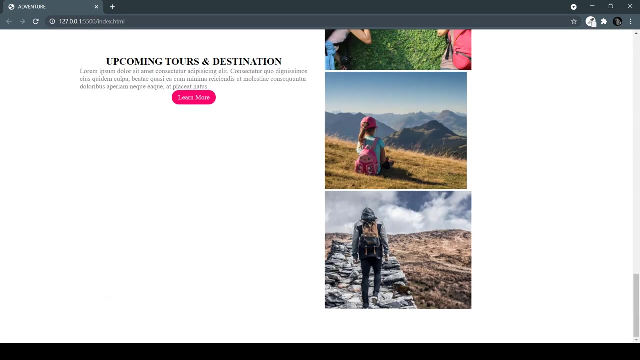 column. let's add a do called image gallery and insert this. we have our gallery and insert this. we have our gallery and insert this. we have our images. set our images for image 3. this images set our images for image 3. this images set our images for image 3. this image for this fire image 6. I can see. 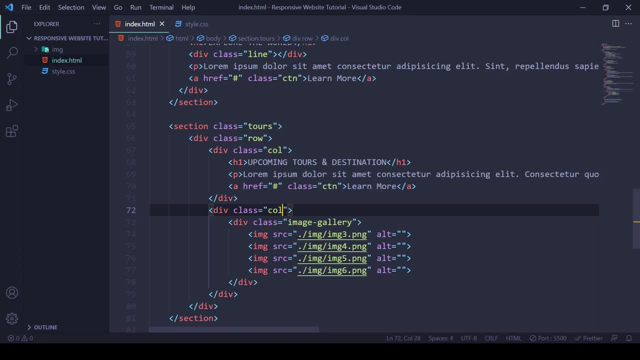 image for this fire- image 6. I can see image for this fire- image 6. I can see all the images here and this beautiful, all the images here and this beautiful, all the images here and this beautiful text and I will add another class number text and I will add another class number. 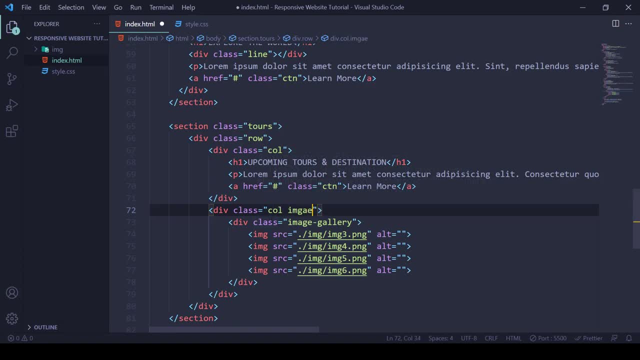 text and I will add another class number: this column right here. this column right here. this column right here. this will be image call so that we can. this will be image call so that we can. this will be image call so that we can target this column and change this text. 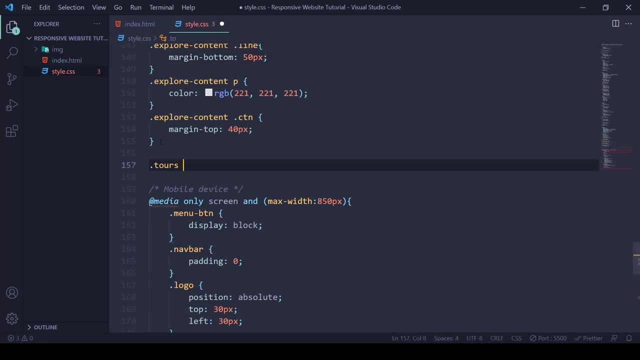 target this column and change this text. target this column and change this text. so now let's open our CSS file inside. so now let's open our CSS file inside. so now let's open our CSS file inside our tours. target our image gallery for our tours. target our image gallery for. 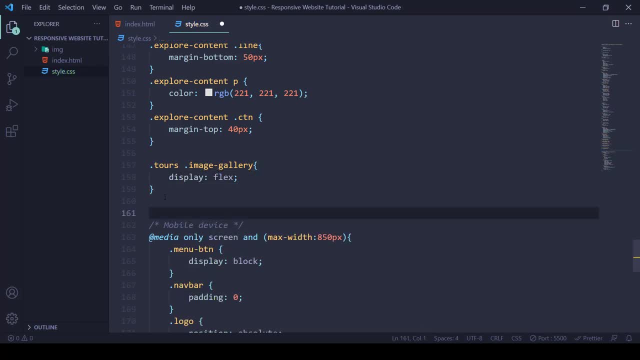 our tours target our image gallery for this: add display flex and inside our this: add display flex. and inside our this: add display flex. and inside our image gallery target our images are: image gallery target. our images are image gallery target. our images are this: add a width at a width of 300 pixel. 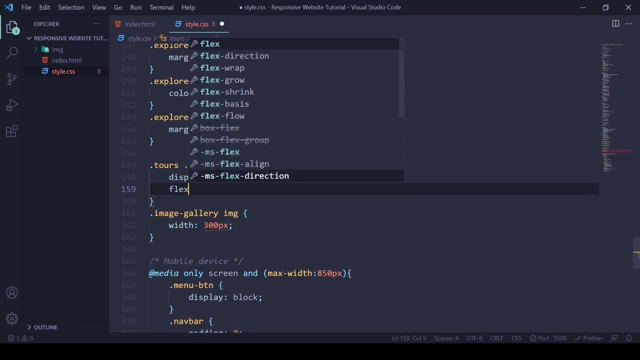 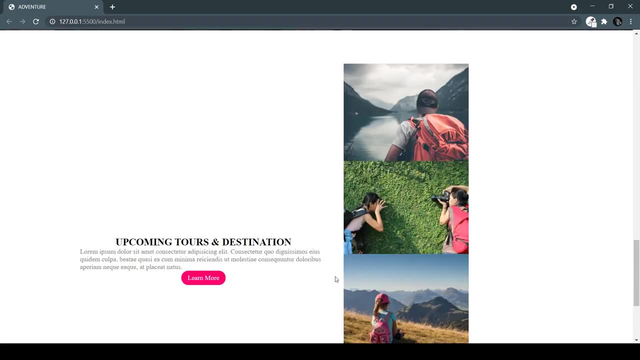 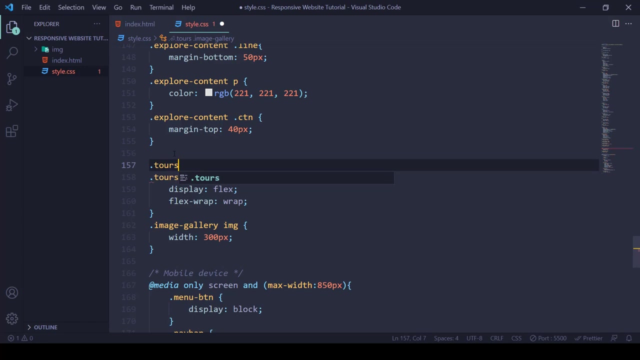 this add a width at a width of 300 pixel. this add a width at a width of 300 pixel. and it here add flex wrap grab and. and it here add flex wrap grab and. and it here add flex wrap grab and. inside our tours and inside our row, or 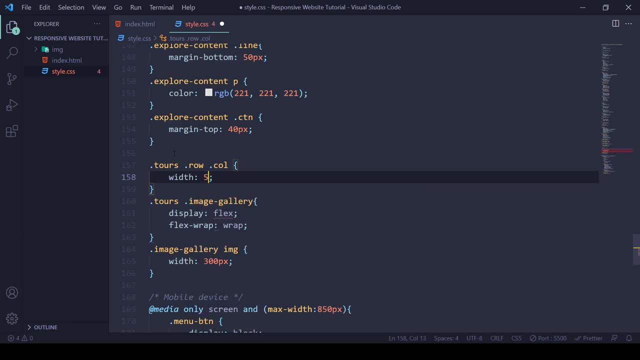 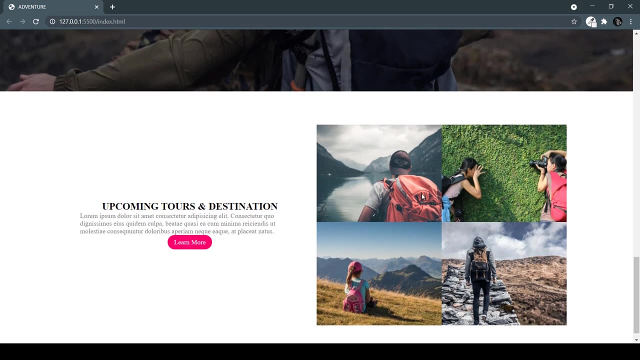 inside our tours and inside our row, or inside our tours and inside our row, or column has a width of 50%. column has a width of 50%. column has a width of 50%. you can see our image gallery here. so for. you can see our image gallery here, so for. 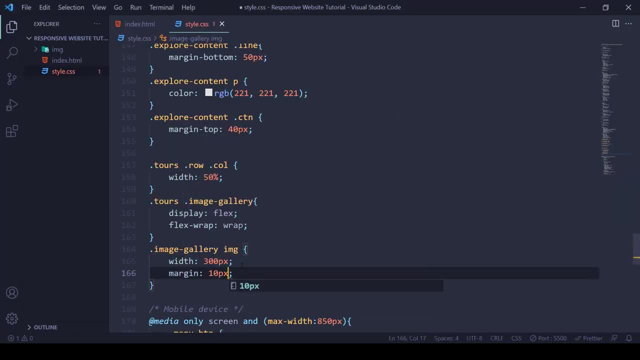 you can see our image gallery here. so for our images, let's add a margin of 10. our images, let's add a margin of 10. our images, let's add a margin of 10 pixel. let's add this image with 250 pixel. let's add this image with 250. 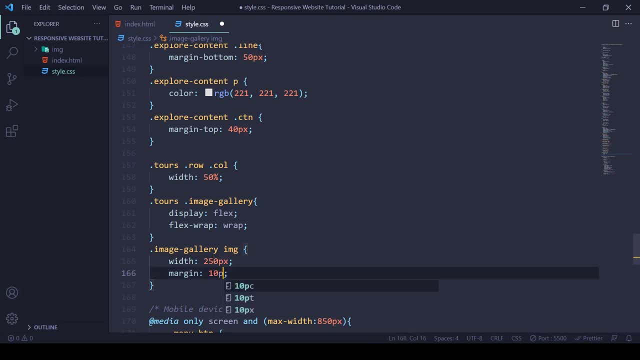 pixel. let's add this image with 250 pixel and a margin of 10 pixel. now I pixel and a margin of 10 pixel. now I pixel and a margin of 10 pixel. now I want to make this image gallery occupy. want to make this image gallery occupy. 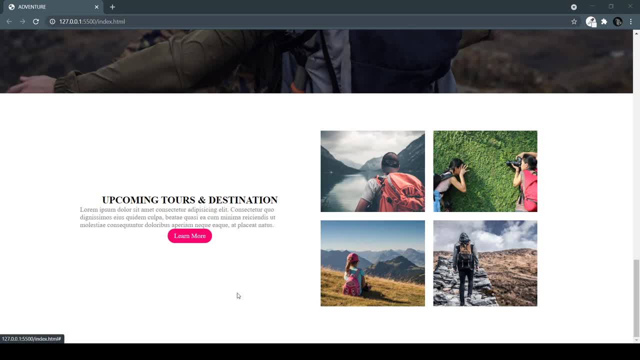 want to make this image gallery occupy more width, and this and this text right, more width. and this and this text right, more width. and this and this text right here, less with here, less with here, less with. so to do that, let's open our HTML file. so to do that, let's open our HTML file. 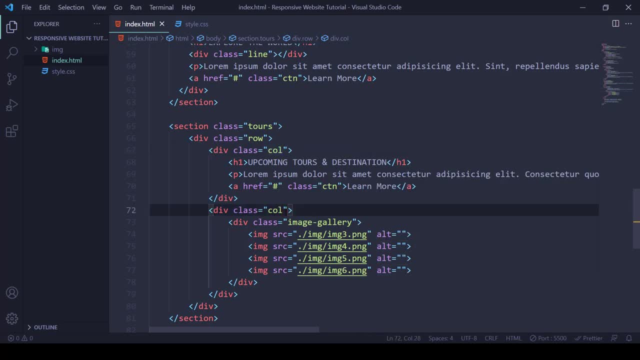 so to do that, let's open our HTML file and that here I will add a class name and that here I will add a class name and that here I will add a class name. content call and it here, image column. content call and it here, image column. 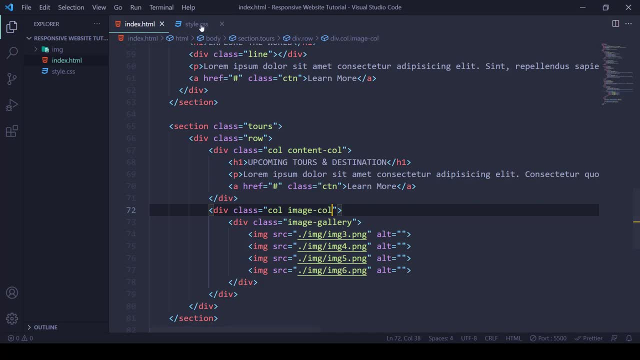 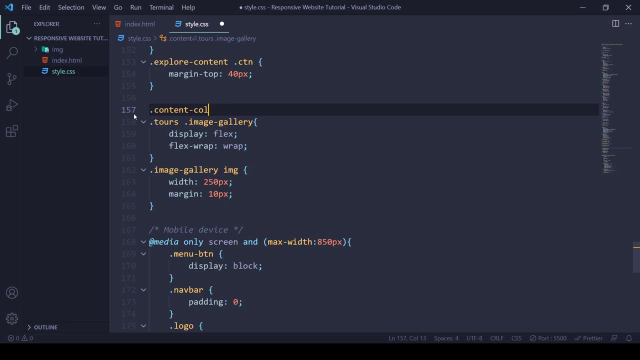 content. call and it here, image column. and inside our CSS file, let's remove this. and inside our CSS file, let's remove this. and inside our CSS file, let's remove this and target our content. call for this and target our content. call for this and target our content. call for this. add a width of 40%. 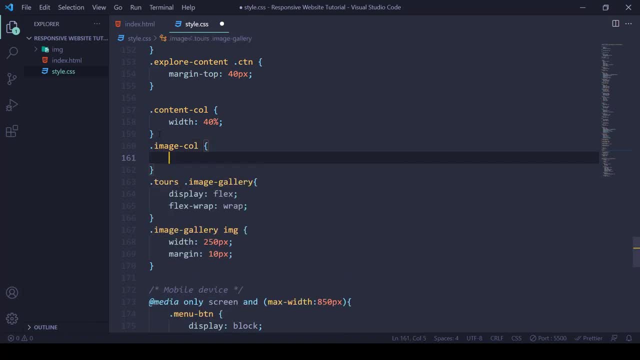 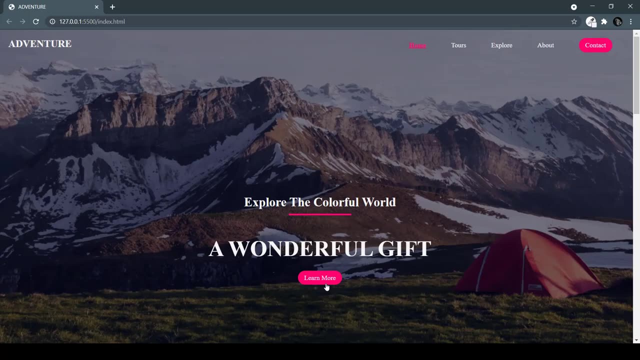 add a width of 40%. add a width of 40%. and for our image call: add a width of 60%. and for our image call: add a width of 60%. and for our image call: add a width of 60%. I can see this is occupying more with so. 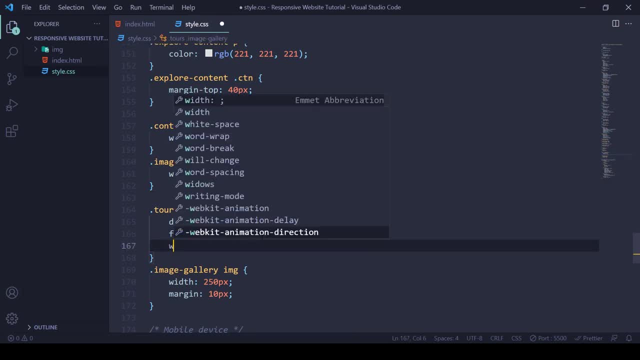 I can see this is occupying more with. so I can see this is occupying more with. so now let's open or CSS file. and for this now let's open or CSS file. and for this, now let's open or CSS file. and for this add a width 100% and align items. Center. 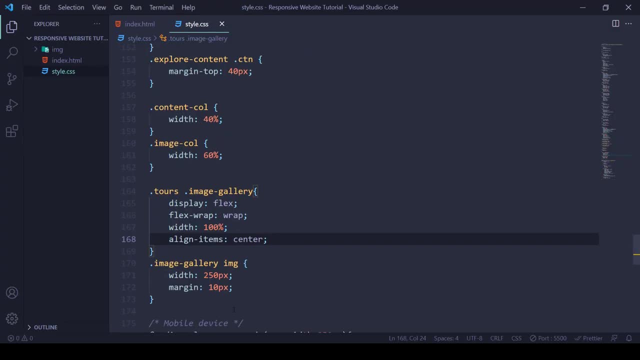 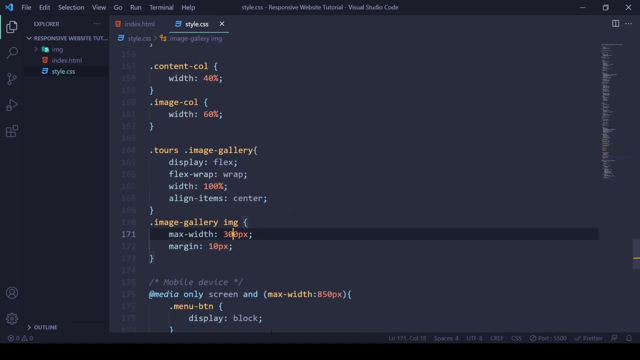 add a width 100% and align items Center. add a width 100% and align items Center inside our image gallery. let's add max inside our image gallery. let's add max inside our image gallery. let's add max width: 300 pixel. I can see our beautiful. 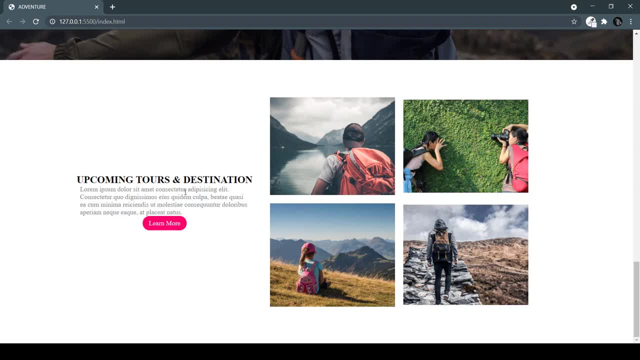 width 300 pixel. I can see our beautiful width 300 pixel. I can see our beautiful image gallery here now. let's now let's image gallery here now. let's now let's image gallery here now. let's now let's style this text so inside our content. 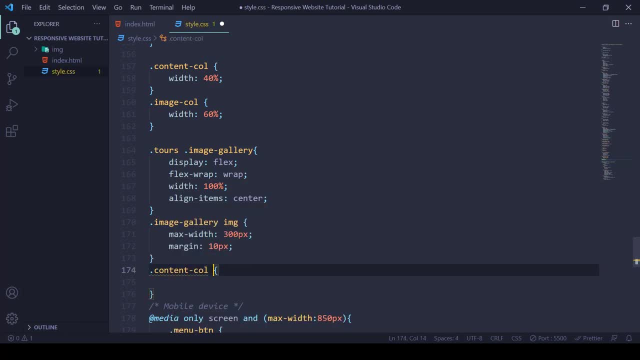 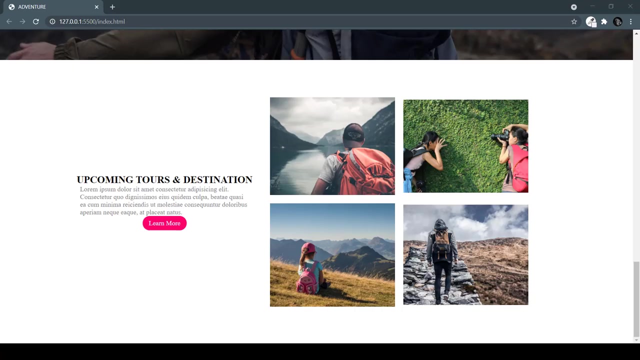 style this text so inside our content. style this text so inside our content. call target our h1 for this font size. and call target our h1 for this font size. and call target our h1 for this font size and 7b min. and color this and inside our. 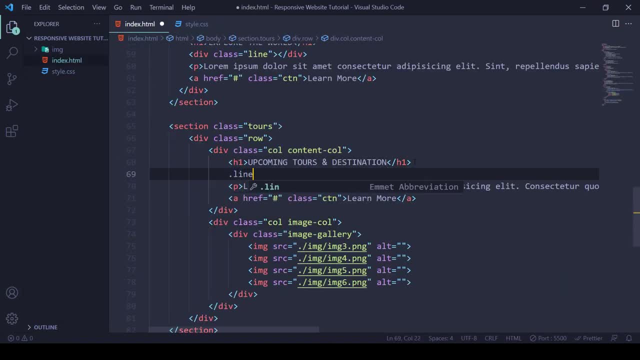 7b min and color this and inside our 7b min and color this and inside our HTML file for this. I will add a line and HTML file for this. I will add a line and HTML file for this. I will add a line and inside your content, call for our line. 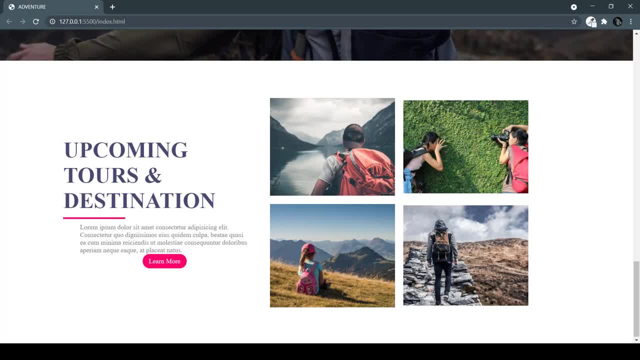 inside your content. call for our line inside your content. call for our line: margin left minus 1 pixel. because we margin left minus 1 pixel, because we margin left minus 1 pixel, because we added margin auto for this at here, so added margin auto for this at here. so 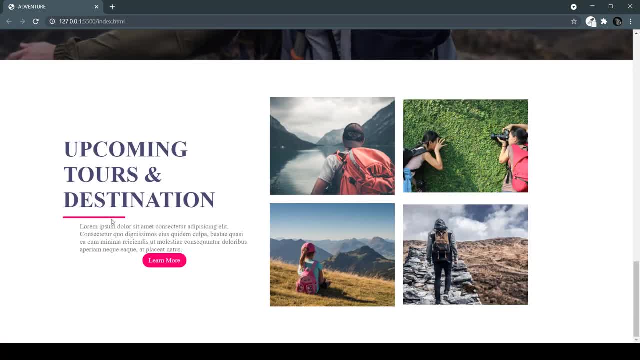 added margin auto for this at here, so this will be in Center now. if we add this will be in Center now. if we add this will be in Center now. if we add margin minus 1 pixel, this will be in the margin minus 1 pixel. this will be in the. 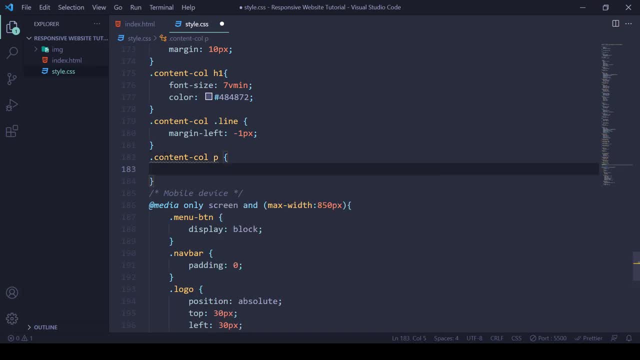 margin minus 1 pixel. this will be in the start, inside our content call. let's start inside our content call. let's start inside our content call. let's target our Peter and for this add padding target our Peter and for this add padding target our Peter and for this add padding zero. and margin: top and bottom: 30. 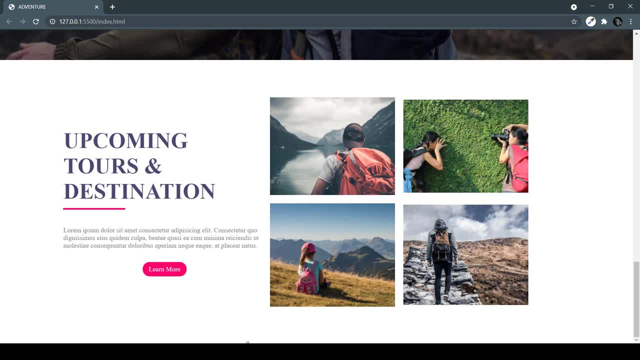 zero and margin: top and bottom: 30. zero and margin: top and bottom: 30. pixel and left and right auto. now let's pixel. and left and right auto. now let's pixel. and left and right auto. now, let's target this, learn more button inside. target this: learn more button inside. 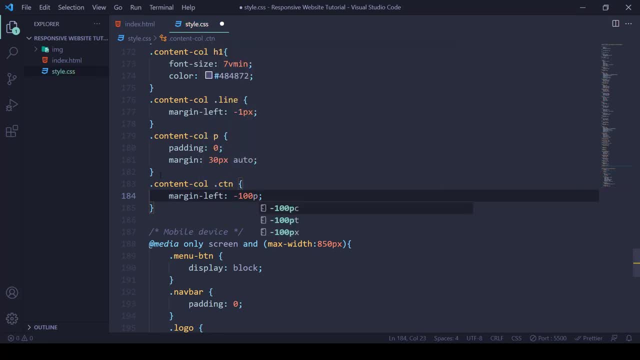 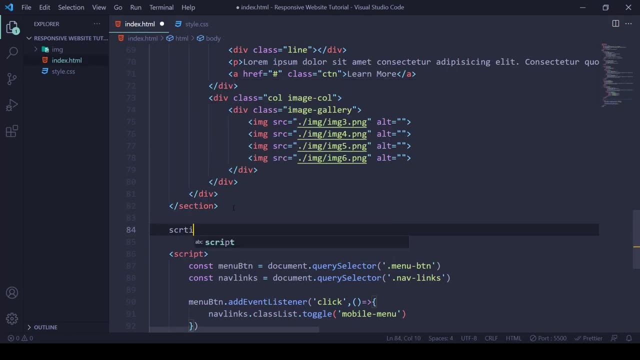 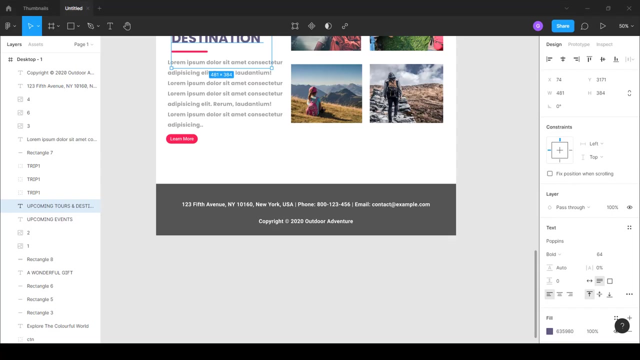 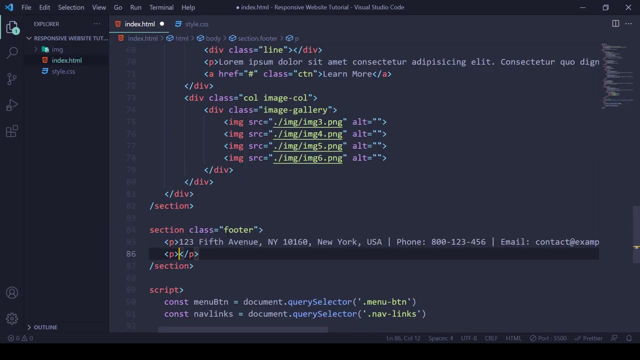 one is 100px. now let's open our html file and after this section i will create another section with a class name of footer, and inside this we have a p tag with this text and another p tag with copyright text. now let's open our html file and after this we will create another html file and after 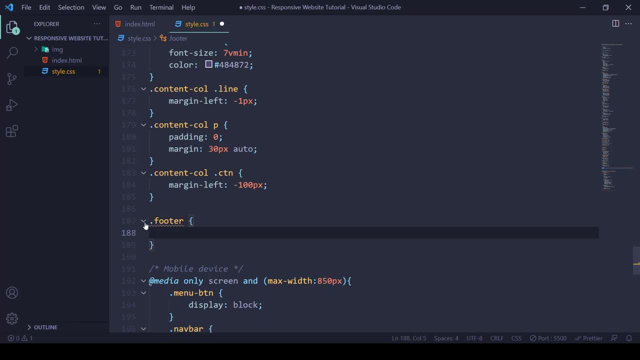 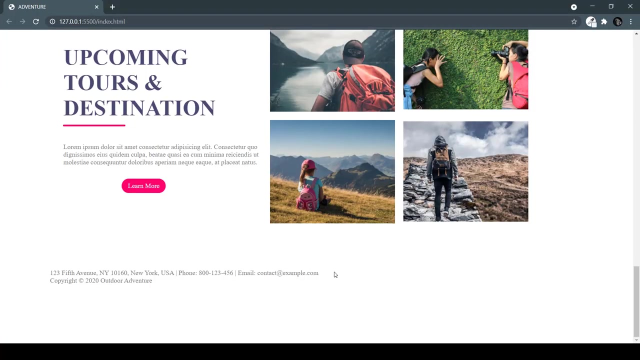 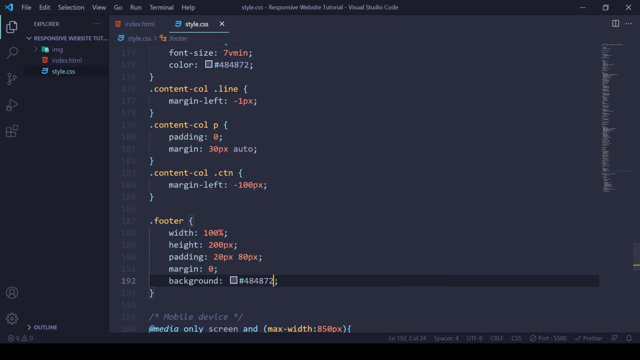 now let's target our footer and for this add a width of 100 percent and a height of 200 pixel and padding top and bottom 20 pixel and left and right 80 pixel and margin zero, and let's add a background of this color and add text: align center. 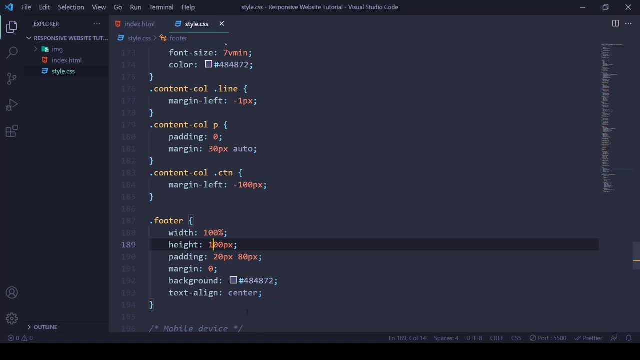 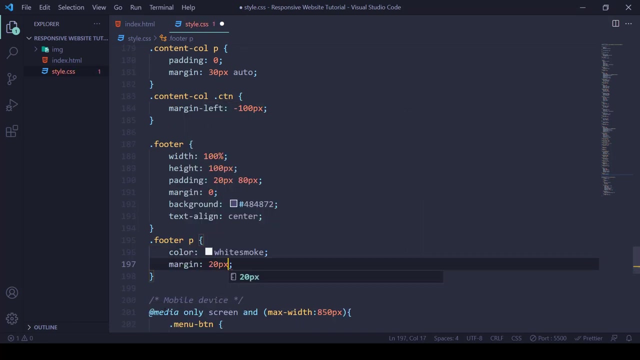 and let's change this width to 100 pixel, then that will be nice, i guess, awesome. so inside our footer let's target our p tag and for this add color: white smoke and margin: top and bottom- 20 pixel, left and right, auto. and padding: top and bottom- 20 pixel, left and right, auto. 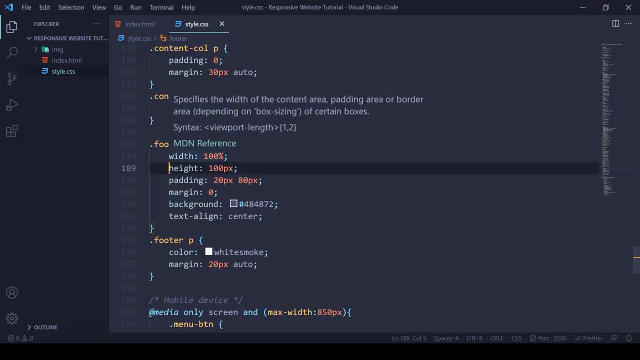 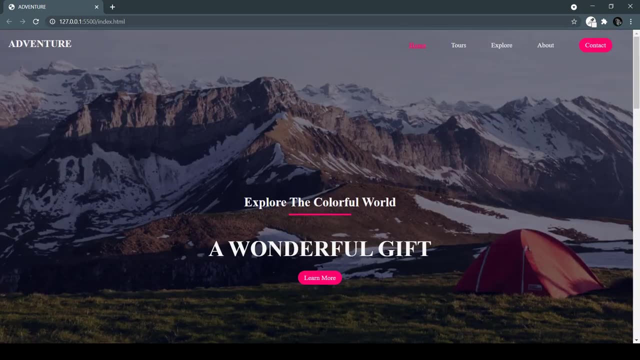 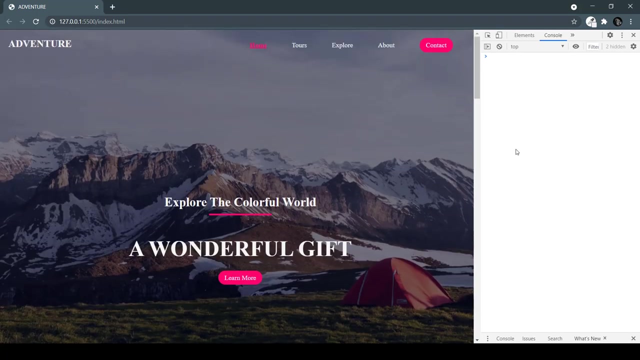 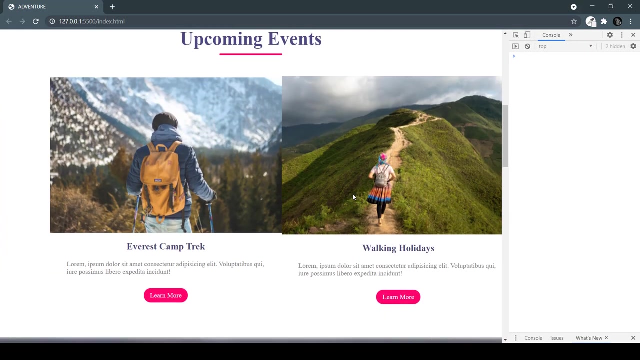 now let's change this height to win height, so that it will occupy the required height. awesome, i can see our beautiful website is completed. now let's make this website responsive. you can see our header section is completely responsive, including this beautiful navbar. now let's make our event section responsive. so to do that. 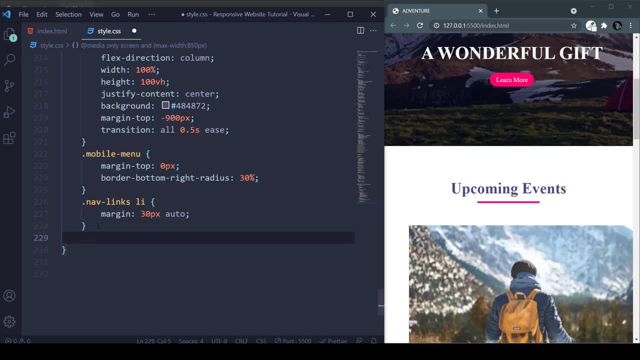 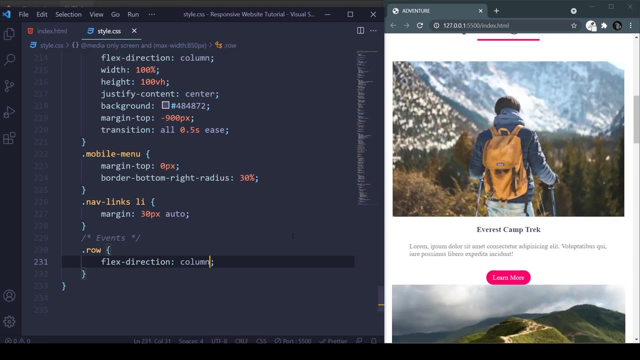 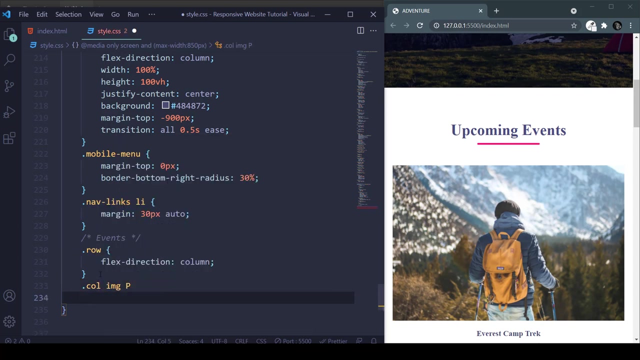 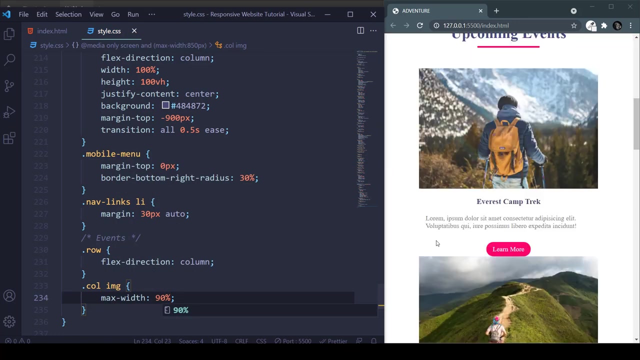 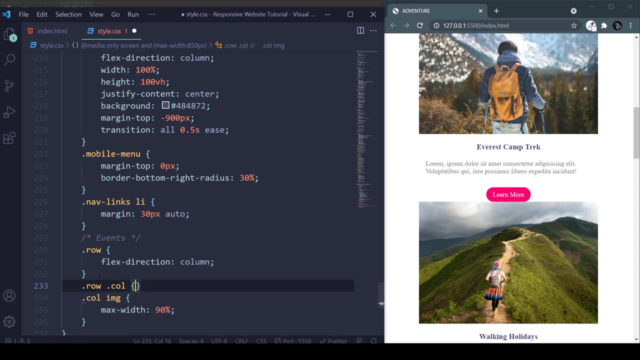 let's open our css file and add here our event section. so for our row, add flex direction to column so you can see our beautiful images here. and inside our column for our image add a max width of 90 percent- awesome. and inside our row for our column add margin, top and bottom, 20 pixel left and right. 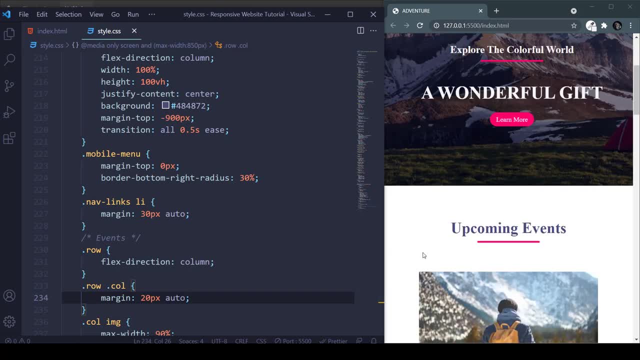 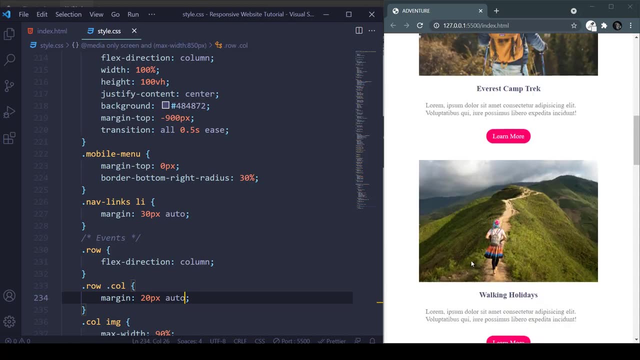 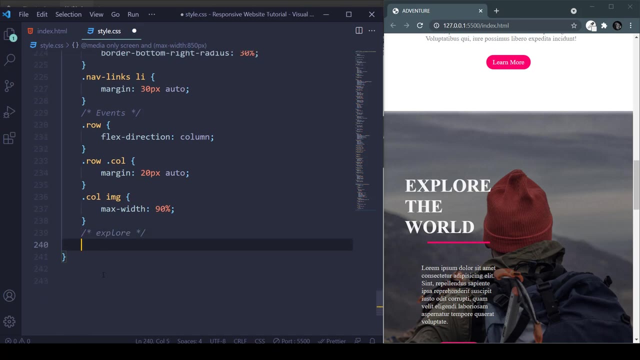 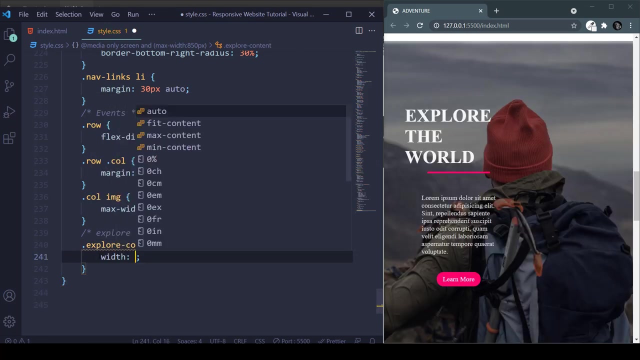 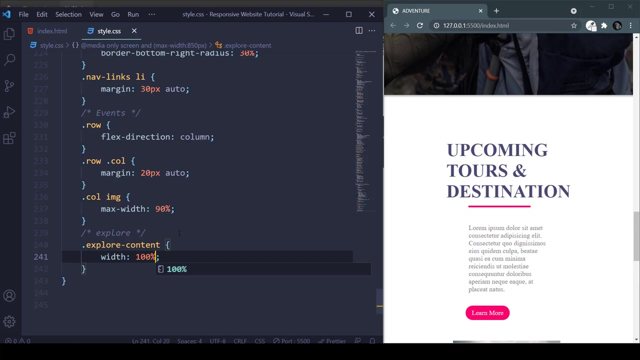 left and right auto. you can see this responsive here. you can see our event section is completely responsive. now let's target our explore section now inside our explore section. let's target our explore content for this add with add width to 100% beautiful. now let's target our tools section inside our. 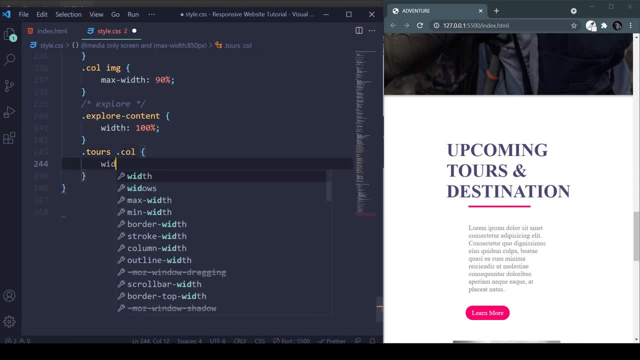 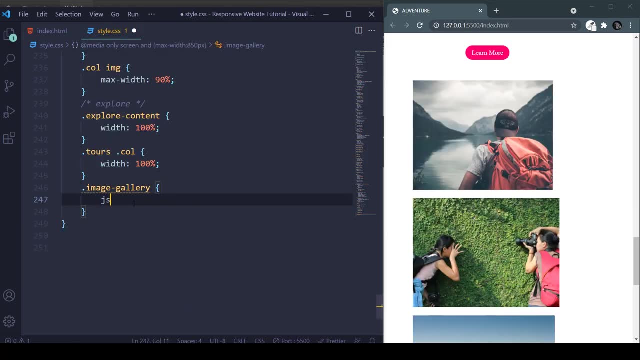 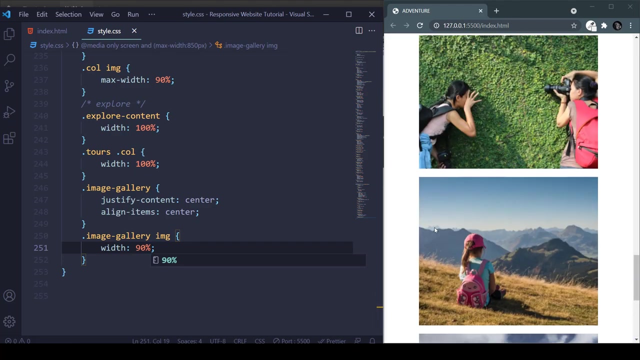 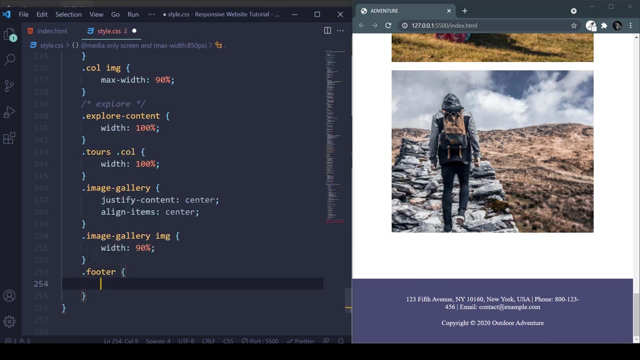 tools. let's target our column for this, add width 100% and inside that, target our image gallery and justify content Center and align items Center. and inside our image gallery, add our image. add width 90 %. I can see our beautiful image gallery here. now let's target our photo section. for this, add padding of 10 pixel. you can see our. 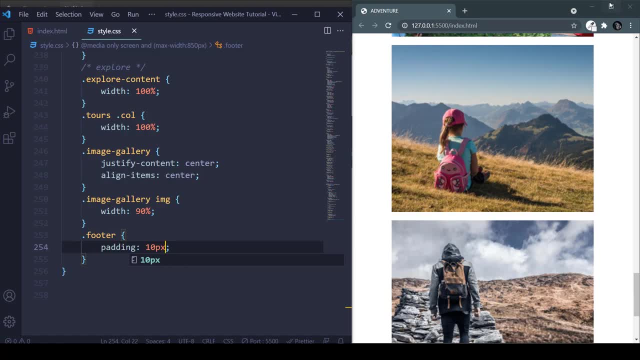 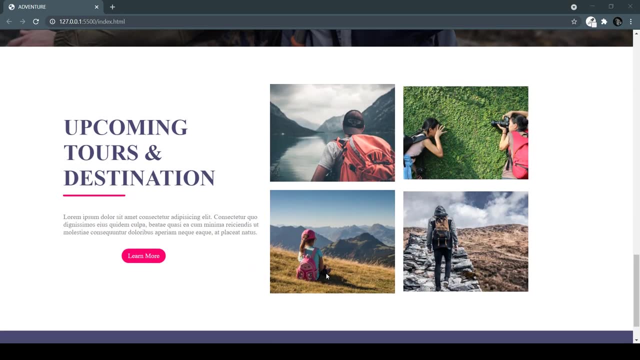 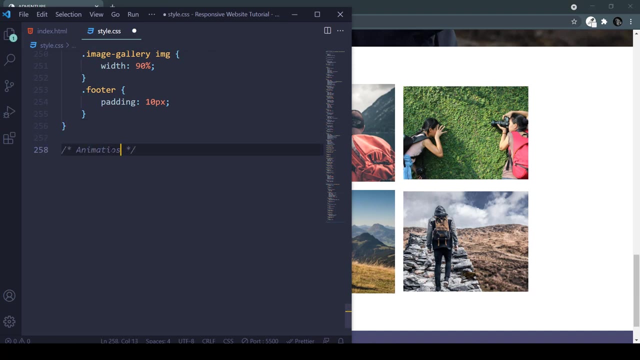 complete. our website is completely responsive and beautiful looking. and now let's add some animations and over-esus effect for our website. so let's open our CSS file and after here leave a comment. animations: let's target our images for this. add a transition for transform. 0.3 seconds is so on our image hover.